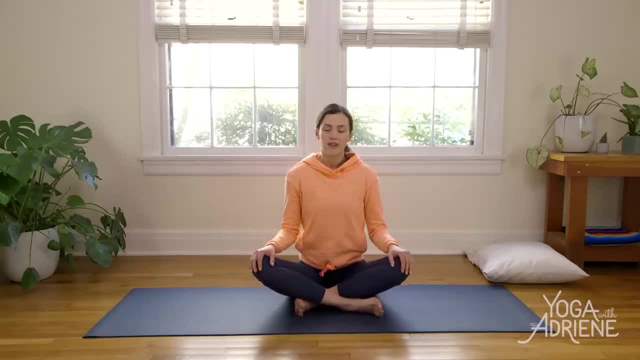 that feels good, Maybe letting go of the day thus far And beginning to notice your breath. I think this is an important moment of the day and of your practice: just allowing, keyword allowing, Just giving yourself an opportunity to drop in tune in, get settled in. 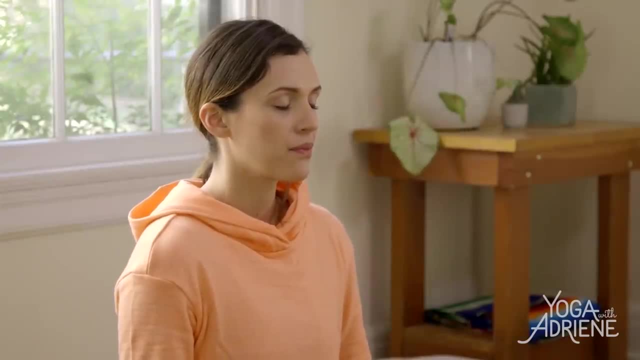 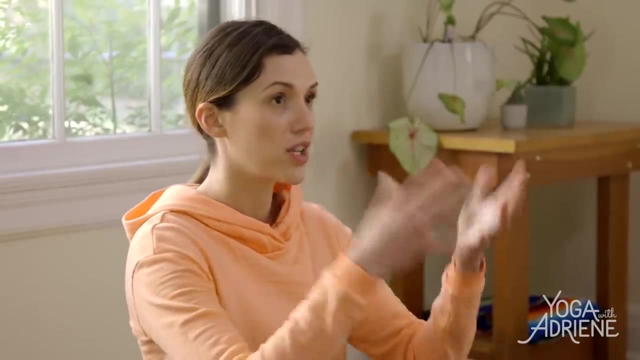 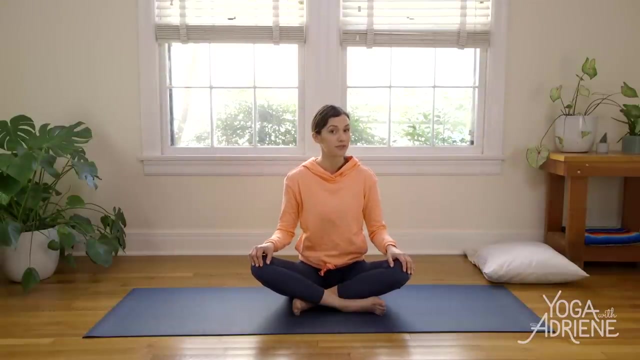 And it's a little different each day, right? The image here is like taking some chalk in the hands or some chalk and throwing it up in the air and watching the dust settle here. That's for you sporty folks, If you're not a sporty folk. 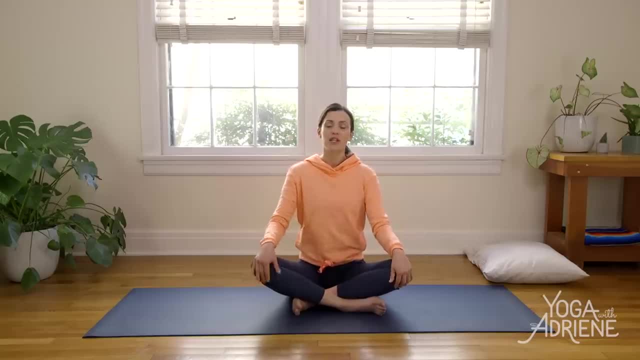 you can imagine glitter being thrown up in the air, Just the idea that it takes some time as it drifts back and forth and down To the present moment. So just give yourself that practice of allowing the dust to settle and just noticing where you are today. 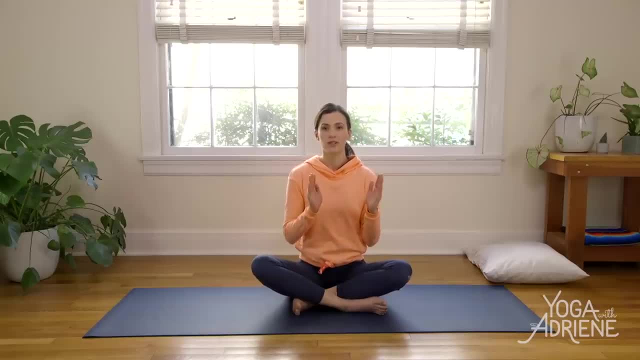 So I know this can be tough because we have oh so little time in our busy lives, but that's what the yoga practice is all about. That's why this video isn't called Runner Stretching, You know, Stretching for the legs. 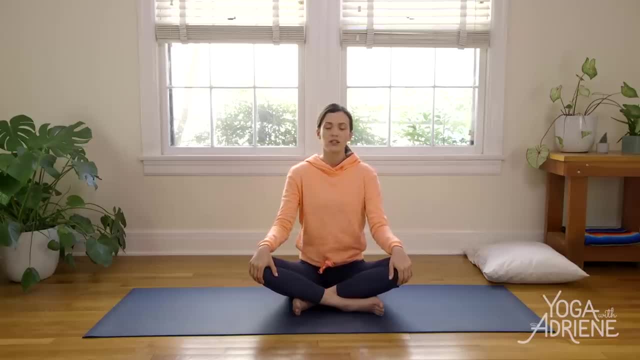 And we're thinking full picture. Hmm, long lasting love with the mind and body. Here we go. So you might notice if you're agitated today or you're really tight. So I encourage you to find soft movement, and that goes throughout today's practice. 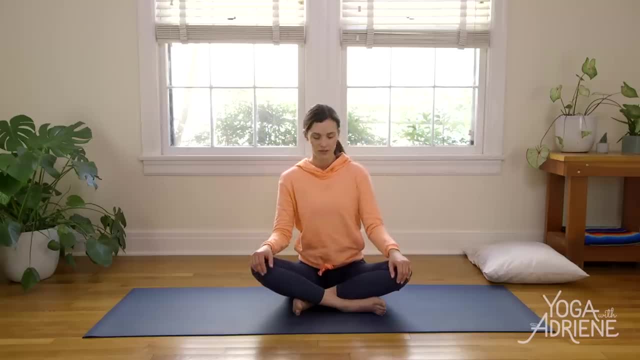 Begin to deepen your breath, if you haven't already. Maybe checking in with some circles with the nose And then, just to kind of kickstart our practice here, we're gonna take three conscious breaths together, So go ahead and inhale in through the nose. 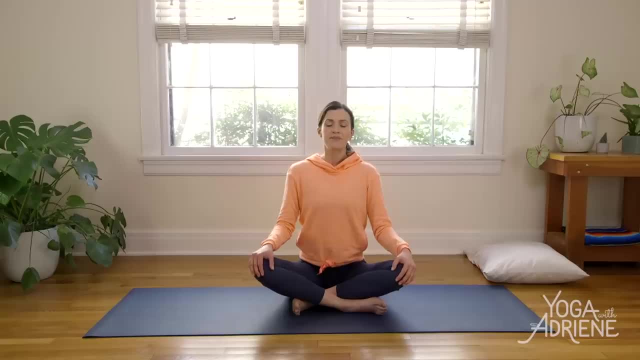 Sit up, nice and tall, Full breath, full, full, full breath in And then just let the exhale go naturally out through the mouth. Great, two more like that Big, conscious breath in, Inhale, fill the lungs. 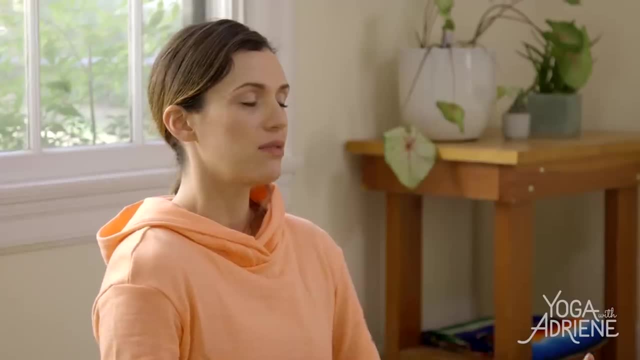 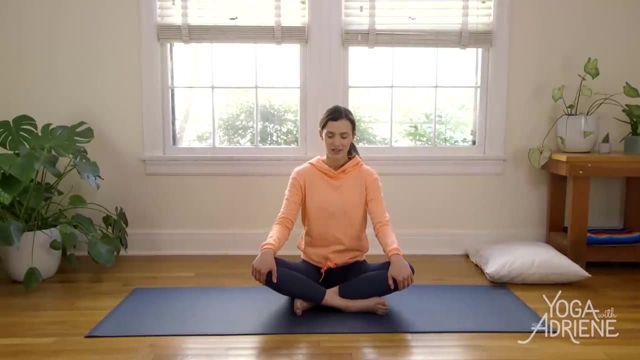 And then on the exhale, it's just very natural to allow it to let go, release. You don't have to do anything. Last time, big breath in, Sit up nice and tall And let it go. Great, So we're gonna take the legs wide here. 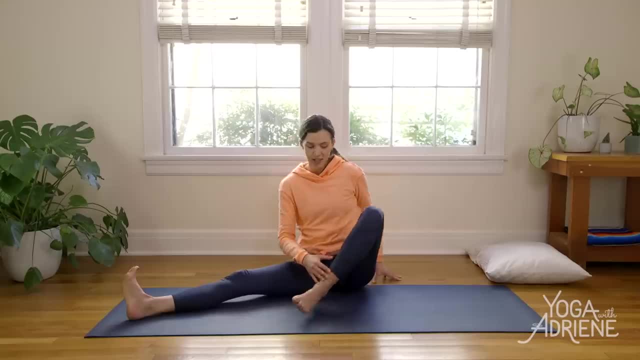 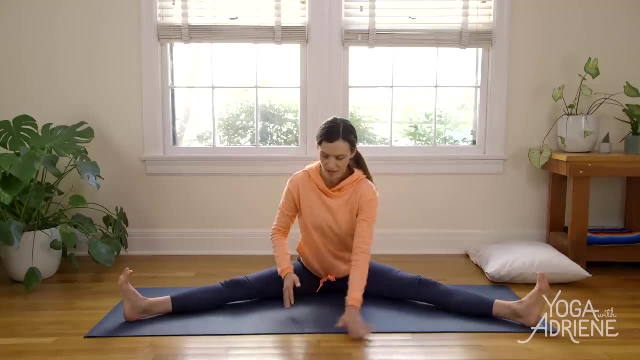 Keep a focus and attention on your breath best you can. Legs are gonna come nice and wide here to your wide, So this will look and feel different for everybody. Right Based on where the muscles are today, how you're dealing with your joints at this point of time. 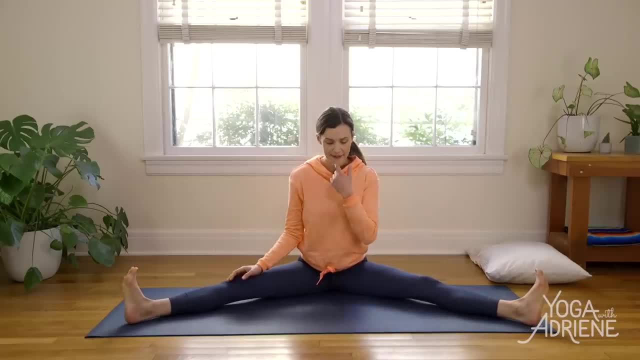 and your energy. So come to a nice wide-legged seat- And again, it doesn't have to be super wide, It can be kind of narrow- And then just see if you can sit up nice and tall here If you're feeling like the spine is rounding hardcore. 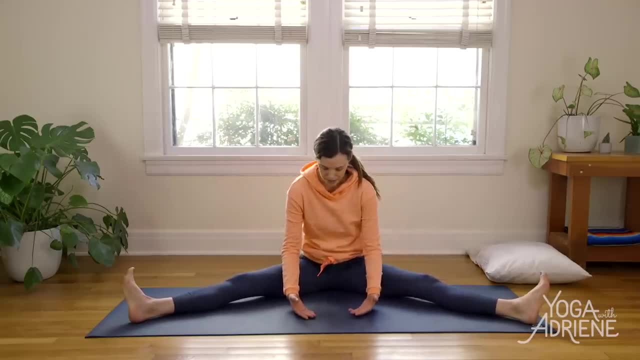 go ahead and sneak that blanket or that pillow underneath And press into the sitting bones. Everyone sit, Sit up nice and tall And then bring the hands to the tops of the thighs, Fingertips in, And we're just gonna gently press the tops of the thighs out. 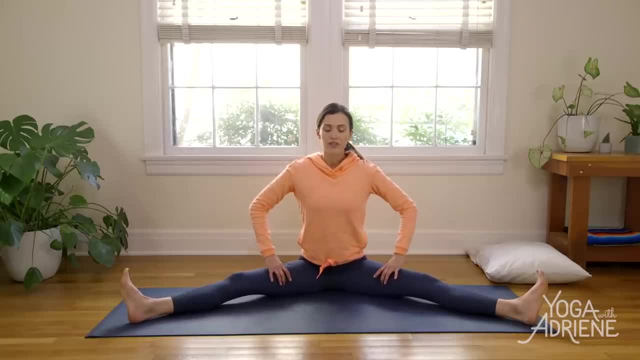 to remind us to find this external rotation. So for some, this will be a piece of cake, And so, in that case, I would recommend that you start really playing with your breath, maybe Ujjayi, And if this is really tough for you, 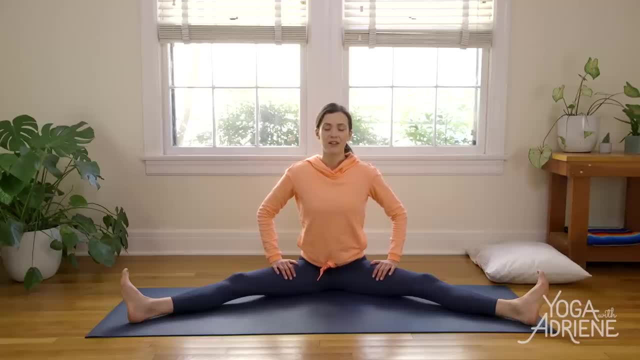 just sit up tall, breathe deep still, Find length through the neck Crown of the head Reaching up towards the sky. Nice little power pose here as we open through the chest, open through the heart, And then release the hands And we're just gonna use the hands to guide the heels in. 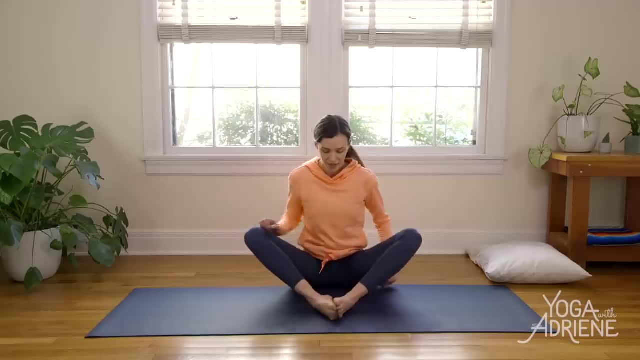 for Cobbler's Pose. So the soles of the feet come together here. We stay conscious, connected through the sitting bones And the hands are gonna wrap around the ankles here. Big loop of the shoulders Forward, up and back. 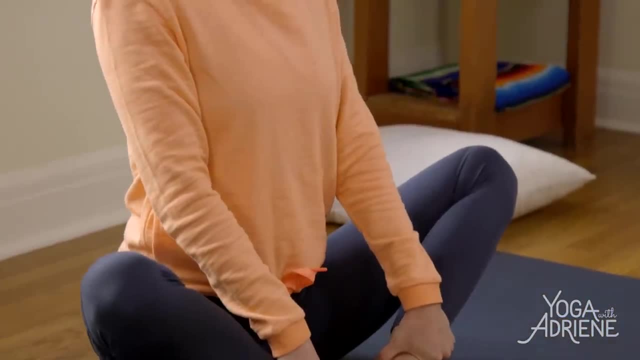 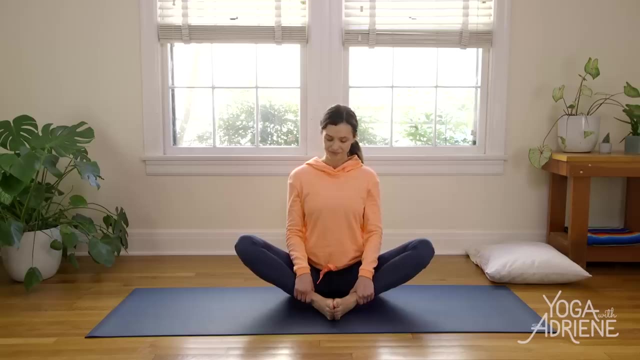 Inhale, in Exhale, glide the shoulder blades in and down the back body. Lots of space between the ears and shoulders here. Then that same external rotation you had in the tops of the thighs just a second ago. try to find that here. 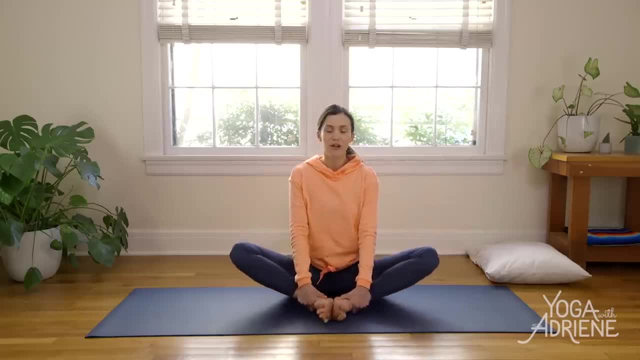 So the hands won't be there, but you can try to ground down through the tops of the thighs, Find your breath Again. So we're not just hanging out here but we're really activating through the quads. So drawing down through the tops of the thighs. 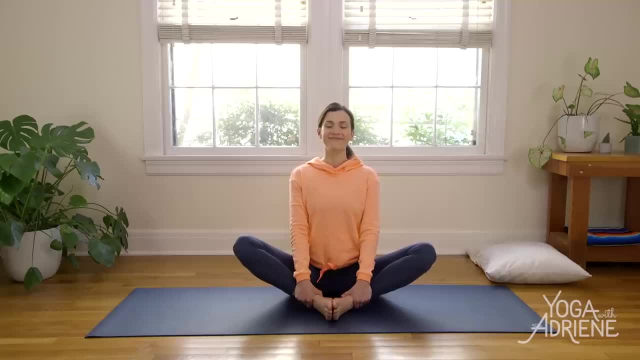 and drawing up through the midline, the plumb line. Again, you might find a little sway here if it feels good, Bring a sense of you softness to these active postures. How can we do that? I think by staying conscious with the breath. 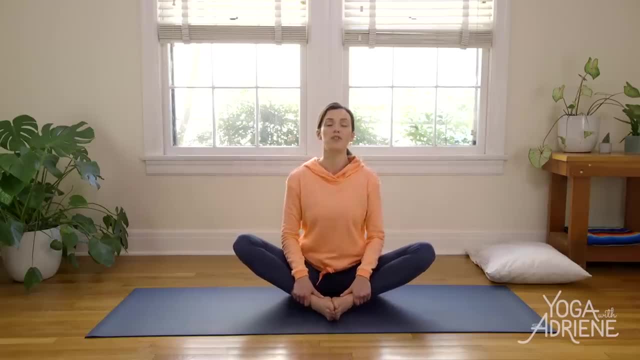 And with practice, Alright. inhale, lift the heart, Think up and over as you send your heart forward beyond your toes. What the heck does that mean? So we're not just rounding forward here, we're keeping length in the spine, elbows grounding down. 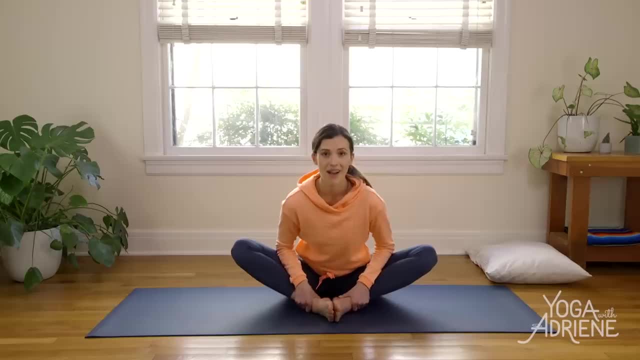 So the image of the heart just reaching forward. My heart will go on And then finally tucking chin to chest, rounding everything forward. Draw your forehead towards your toes, Doesn't even have to come close. Breathe, Breathe deep. 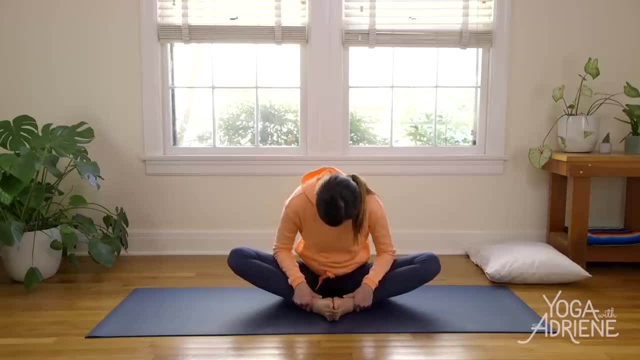 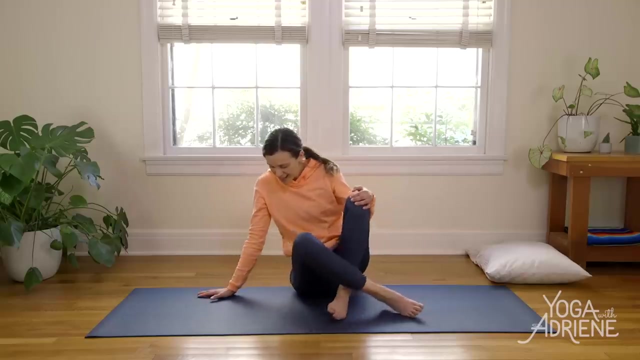 Then anchor through your sitting bones once again to roll up. Tuck the chin to the chest. Should feel good, Nice and slow. Why rush? it Feels good, Lift the heart And exhale, release. Awesome work. Alright, we're gonna come on to all fours. 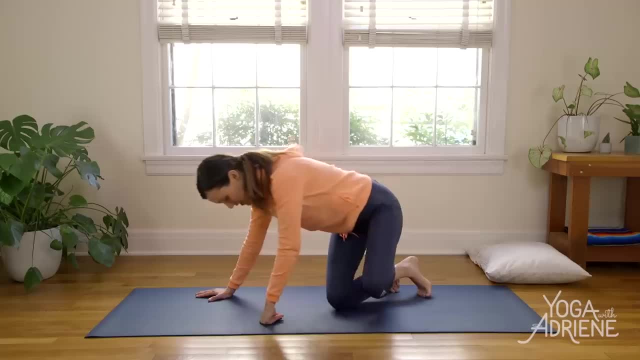 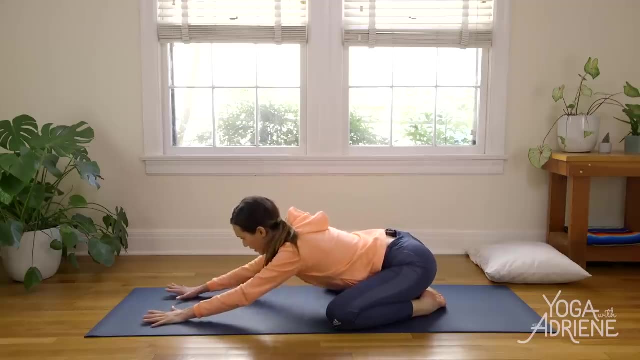 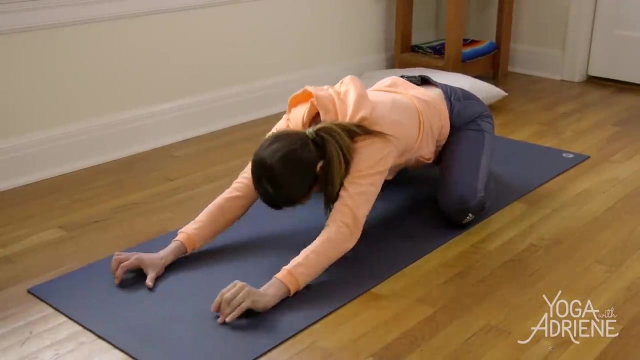 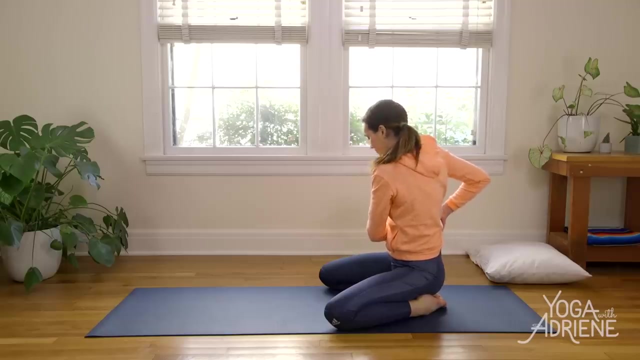 And into extended child's pose. yay, Knees as wide as the yoga mat, Big toes to touch. Walk the hands out, Melt your heart down. Bring your attention, your awareness, back to the breath. Close your eyes. See if you can make your inhalations longer, smoother. 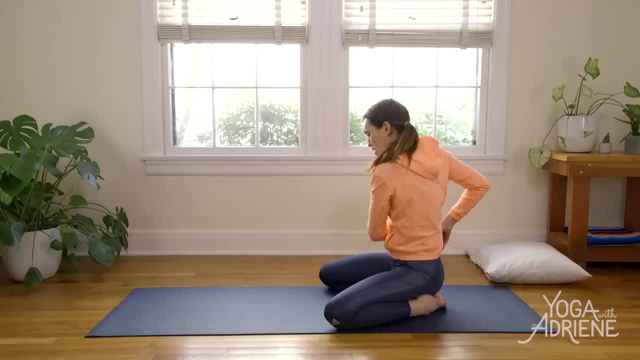 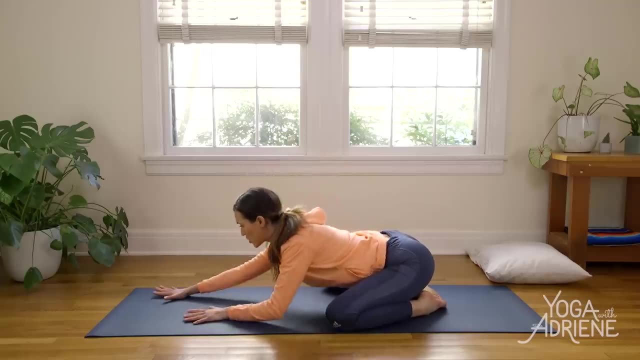 As well as the exhalations, nice and long, Really pushing out all the air. If you are a runner or a wannabe runner, you will soon learn that the relationship with your breath is key. Dreams are just an opportunity, I believe, to receive greater. 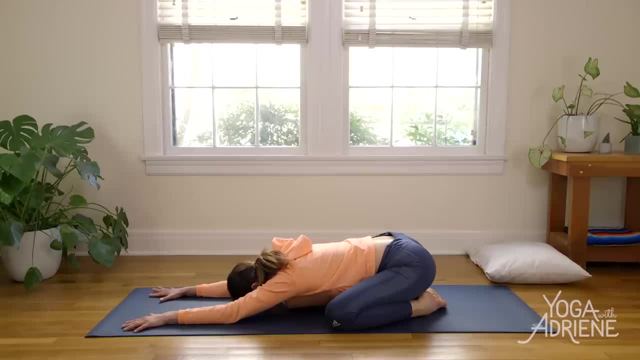 Black Time, Something you'll need to take a step for in a remain strong human condition. Who you are is not necessarily true. Live your life the way you want. Live the way that you think you want. Live your life in flush with your time, to your heart and. 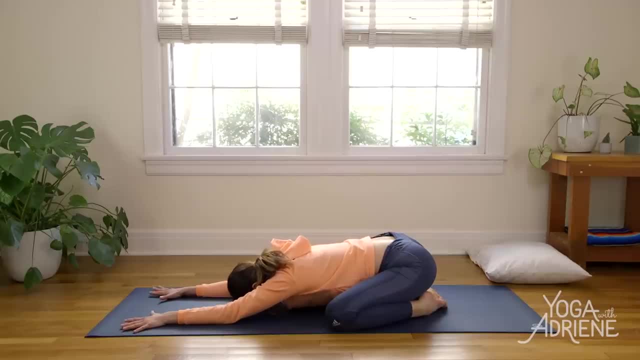 the things you feel can be necessary. Look for something you can do. You can do anything. Be something, Be sound, Mind, Think, Think And then, slowly pressing into the palms, We'll walk it back up. Come to tabletop position on all fours. 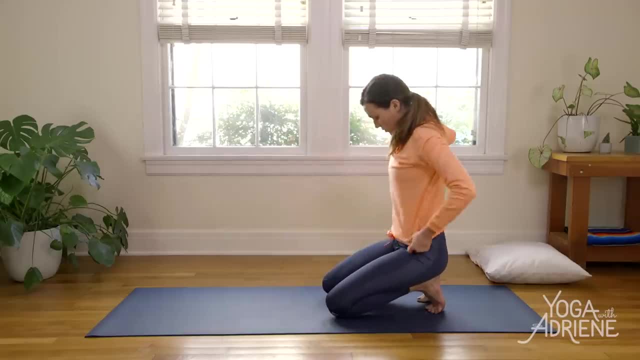 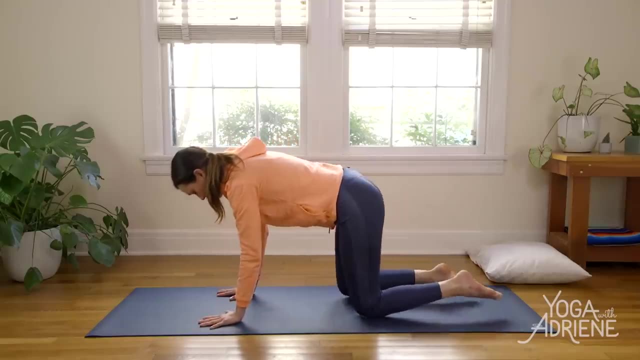 Knees underneath the hip points, Wrists directly underneath the shoulders. Take a second to press away from your yoga mat with the palms, Then we'll curl the toes under on the right foot and slide it back. little calf stretch here, as you gently saw, front to back. 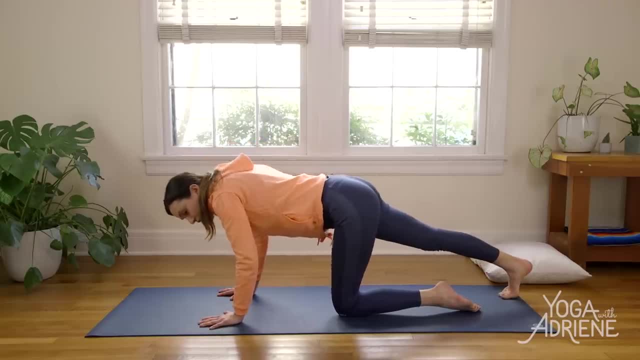 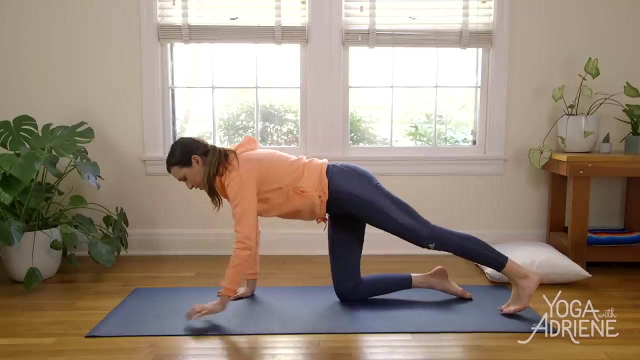 So, gentle, rock front to back Again. no collapsing here, but pressing away from your yoga mat with the palms. Try to press into your right pinky toe, Keep breathing And then switch. Curl the left toes, send it back. Same thing here. 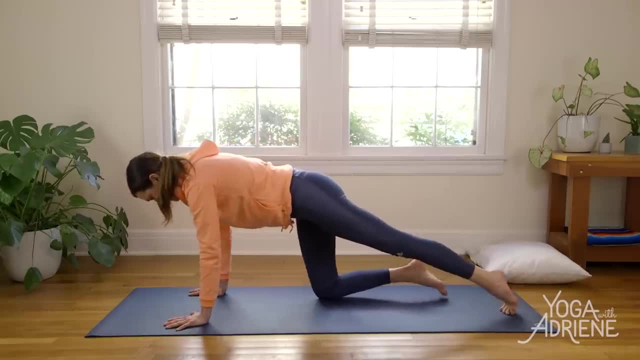 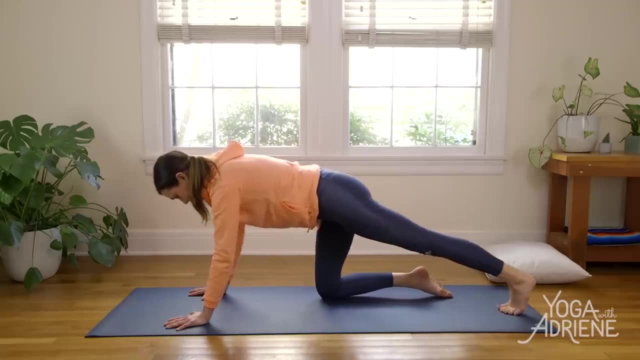 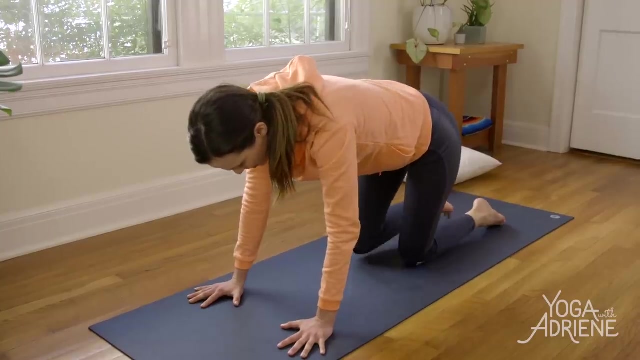 We'll walk forward a little bit, Try to press into that left pinky toe And then roll it back into center. awesome. So now we're gonna send the right toes out, Lift the right foot up, Lift from the right inner thigh. 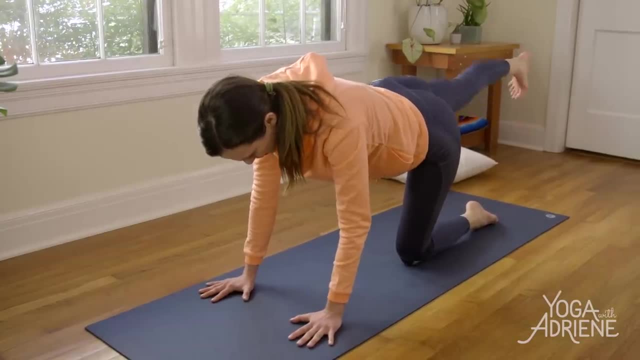 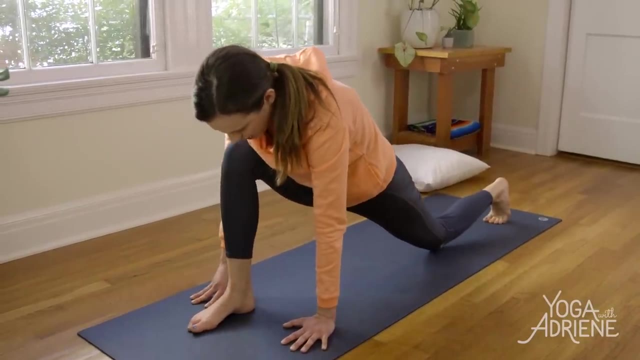 And then just gentle pulses here, Then release, bend the right knee, step it all the way up into a nice low lunge, Walk the left knee back a little bit here. Check to make sure front knee is over front ankle. so it's not going past. 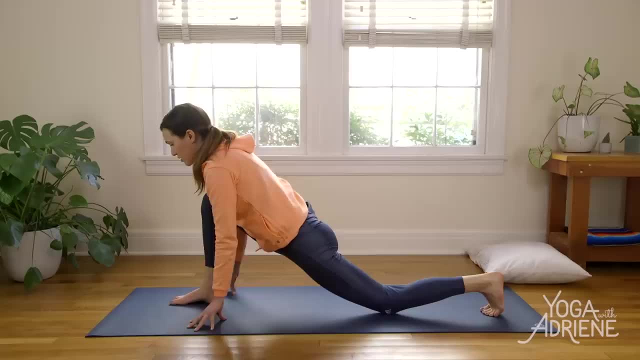 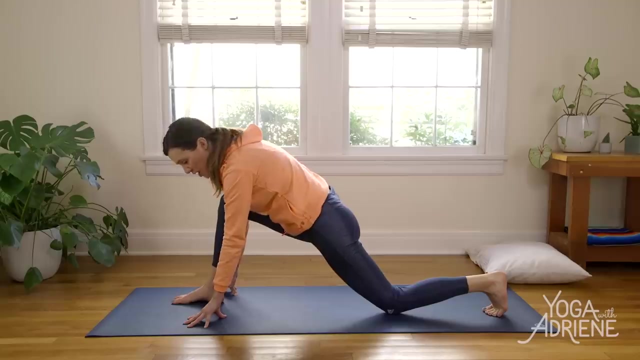 Then find your foundation and breathe here light on the fingertips. You might loop the shoulders, Find length through the crown And then imagine my heart will go on again here, so nice and open in the chest, not collapse. This is very common and very normal, natural. 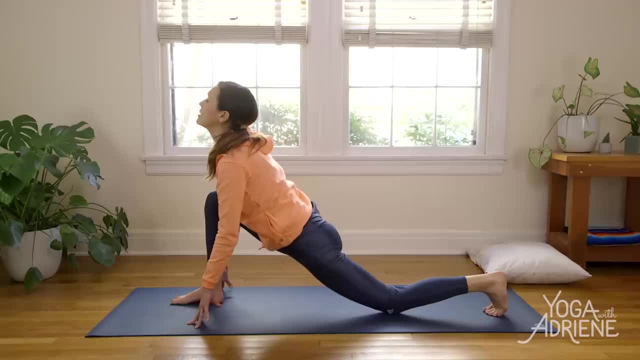 So we're wanting to open this up right. This is definitely gonna help our running game. Keep breathing here. Pull the right hip crease back Again. if this is a problem, it's okay. It's gonna be okay, It's gonna be okay. 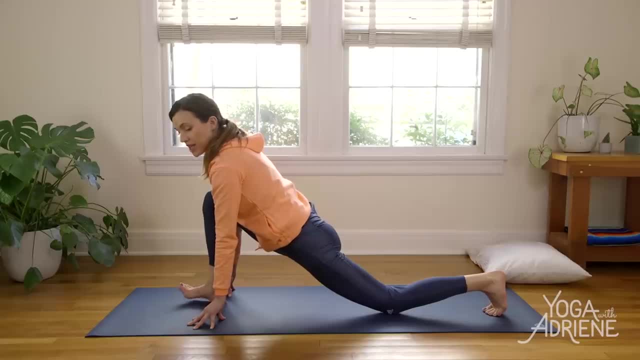 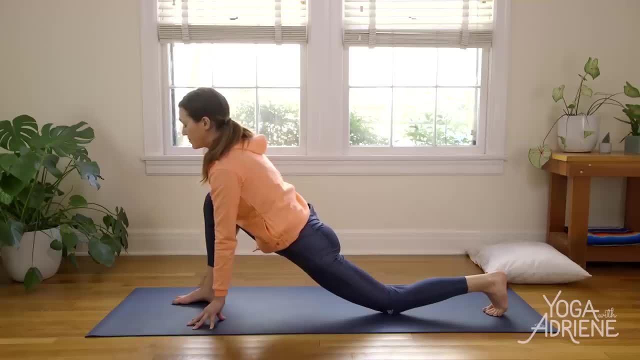 Any big, big inhalations all the way down And then exhale all the way up and out. So the first step you know often is just kind of learning the shapes and then it's really up to you to kind of go deeper. 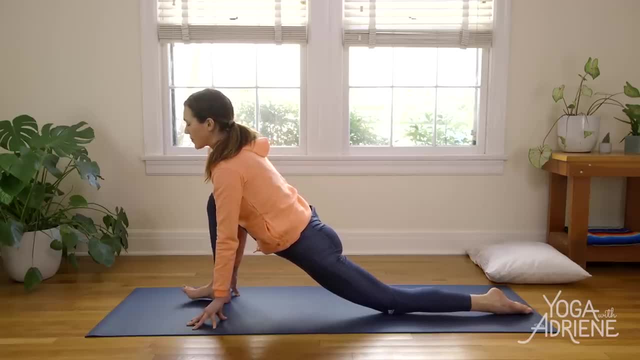 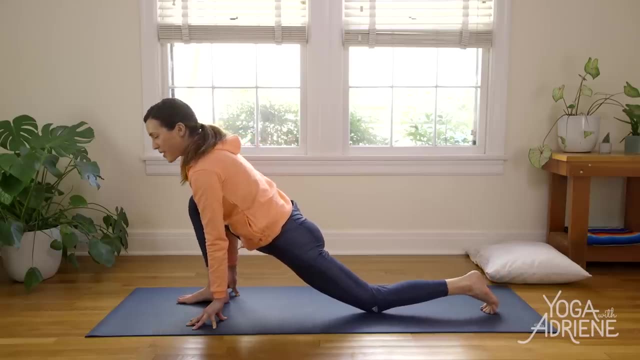 and take care of your body and to apply the pranayama practice. Here we go. Curl the left toes under. if they are not already, We're gonna lift the hips up and back, rocking onto the right heel. Big runner stretch here. 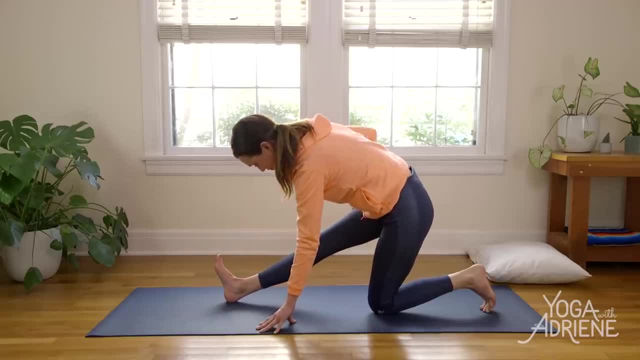 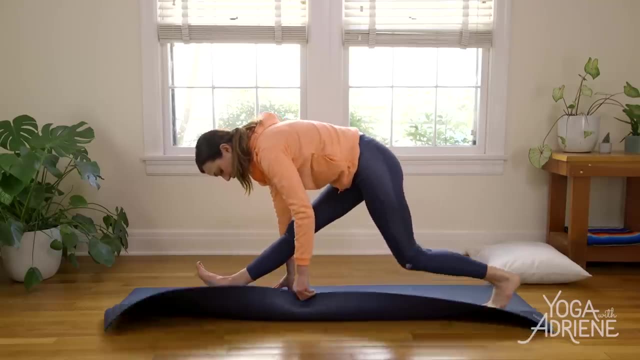 So pulling back through the top of the right thigh bone, And then you can uncurl the back toes if it feels better. If the knee needs a little padding here, it's always a great idea to nurture that, maybe by flipping the mat, rolling the mat if you need. 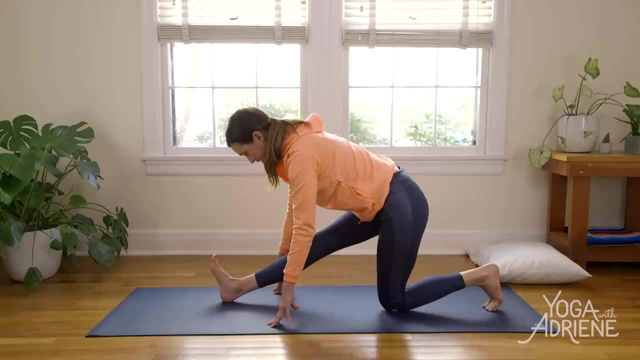 Right toes up towards the sky. Here we go. My heart will go on. Find that length, Inhale And then exhale. fold Chin to chest, Then really articulate through the right foot here. Spread the right toes And then we're gonna roll through that right foot. 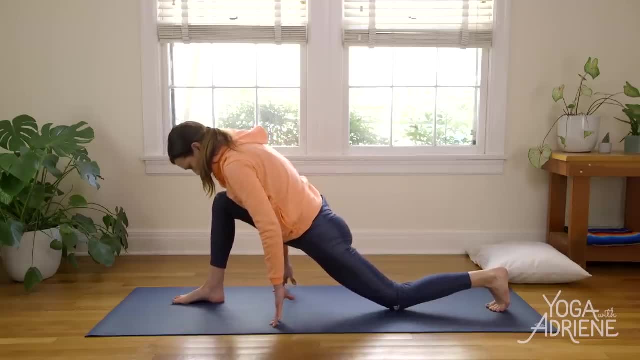 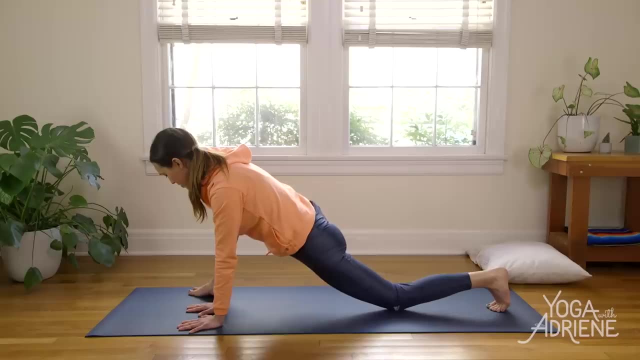 nice and slow. Great, From here we'll bring the palms to the mat on the left side, And we're just gonna give ourself a little bit more space by walking the right foot out. So now we're coming into a lizard variation. 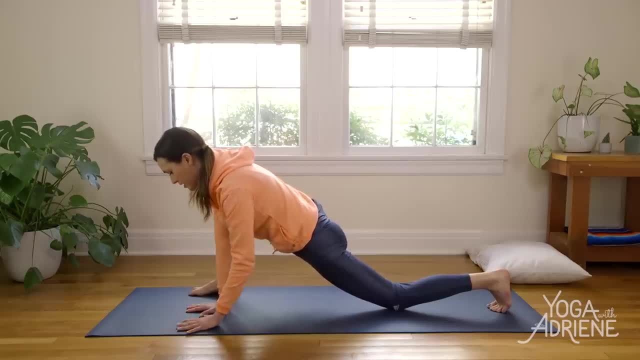 This can be one tough cookie if you're tight in the hips. So breathe deep here For now, right toes pointing forward. If you want more strength today, of course you can lift that back leg, But in honor of today's kind of 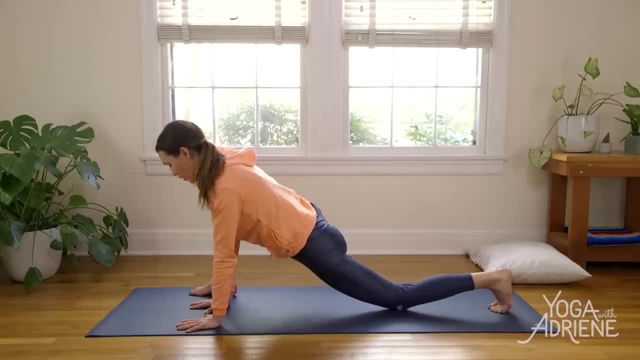 deep and yummy, yin-like theme. I'm gonna keep my back knee lowered, but you're welcome to lift, Take a deep breath in here, Find that extension through the heart And then exhale. Maybe we find ourself coming onto the forearms here. 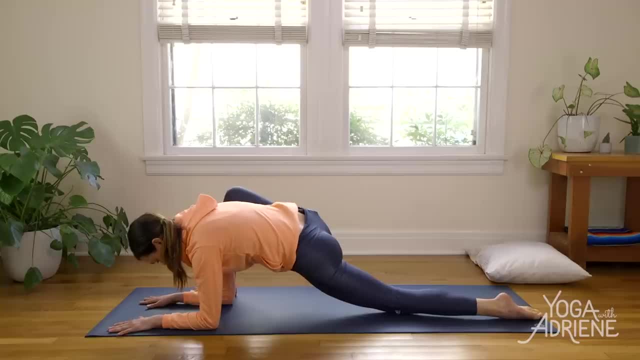 Maybe you find yourself releasing the top foot And then, nice and easy, take it nice and slow. I'm just gonna walk the right toes out towards the sky, Towards the right edge of my mat. Hmm, I'm gonna be here for some solid, yummy breaths. 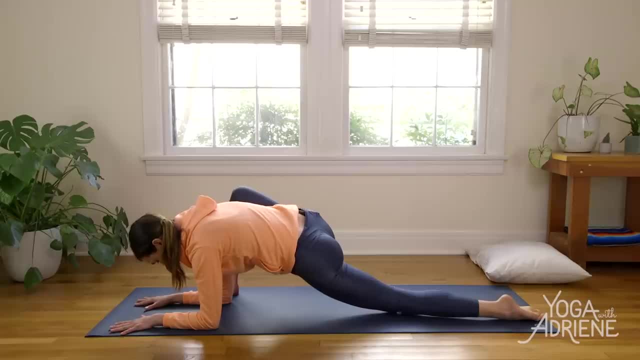 So stay present. Maybe you close your eyes, Notice the sensations as you inhale And exhale. Take one more juicy breath in and out, Then connect to your center, your core, as you press into the palms And slowly, mindfully walk it all the way back. 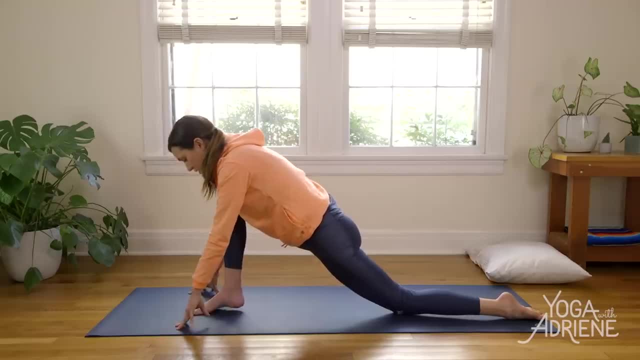 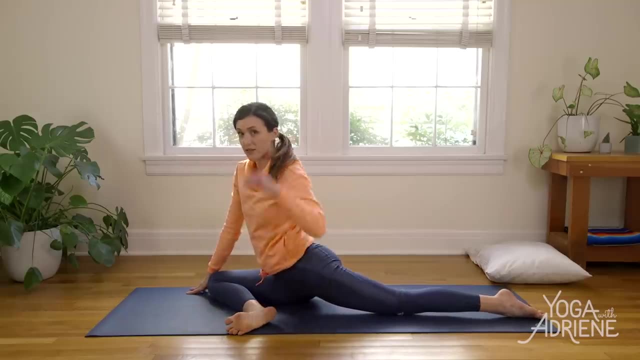 Okay, we're gonna take this right foot all the way over now, Nice, and slow, Slow and steady wins the race Coming into our One-Legged Pigeon. Keep a little awareness, or a lot, rather, of awareness, in the right foot. 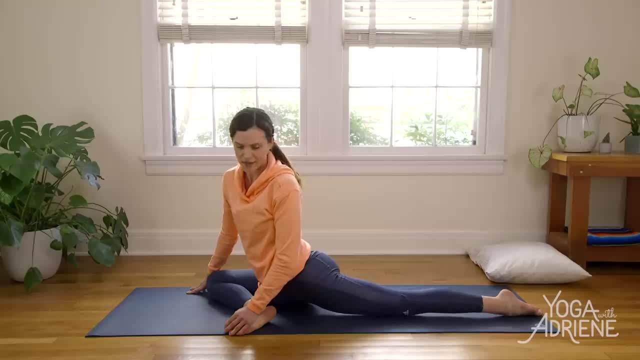 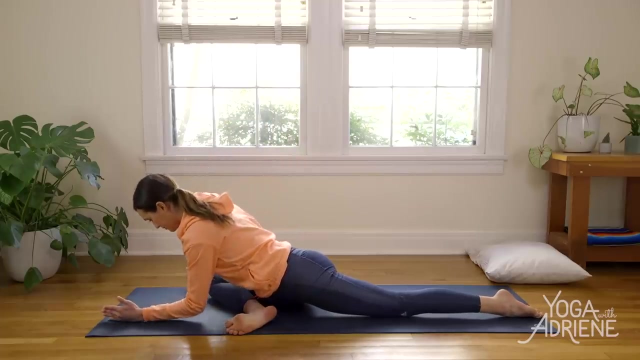 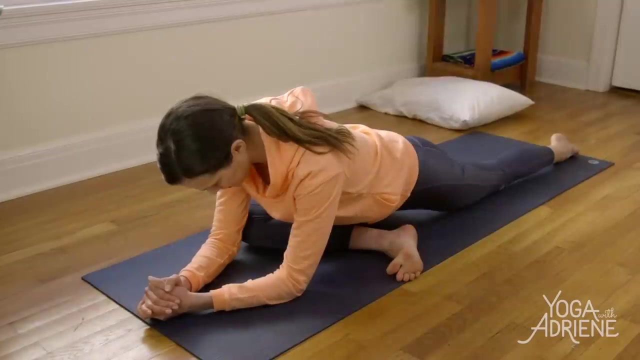 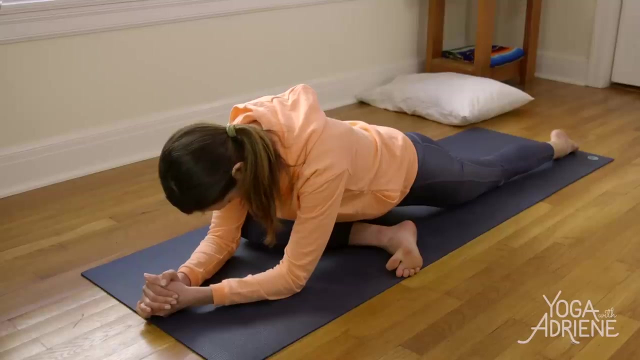 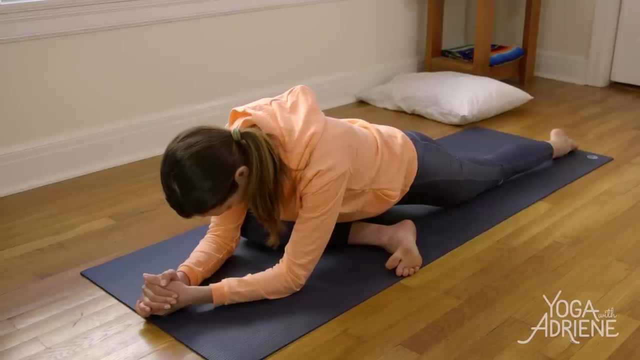 Keep the top of the back foot down- Excuse me rooting strong- And then here we go, Loop the shoulders, find length, Breathe, And then maybe taking it forward. And then here we go. So we're staying in the postures a little bit longer today. 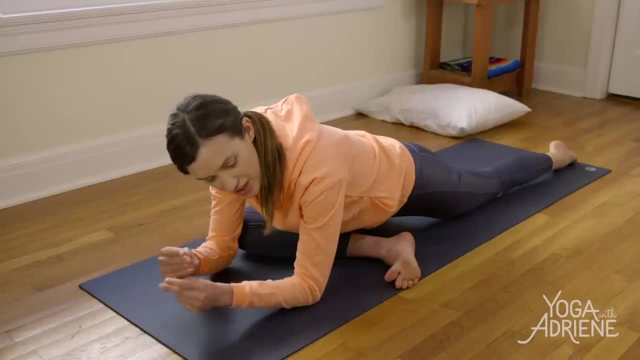 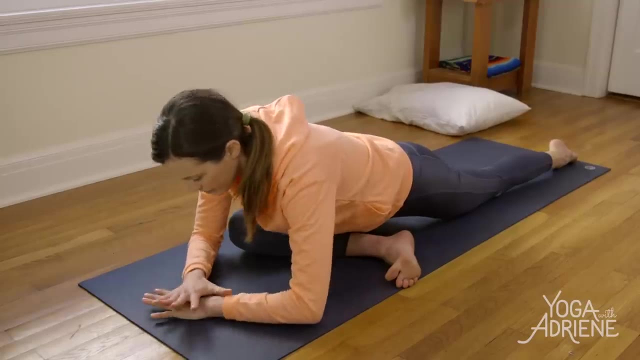 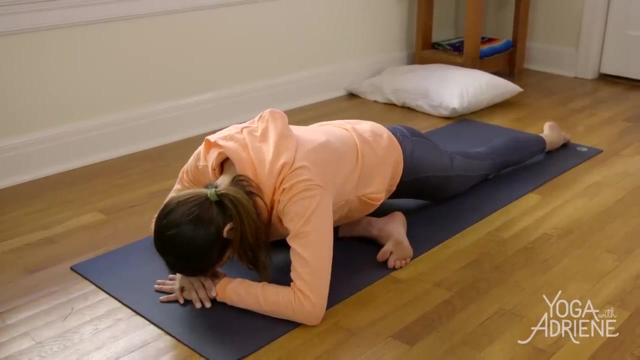 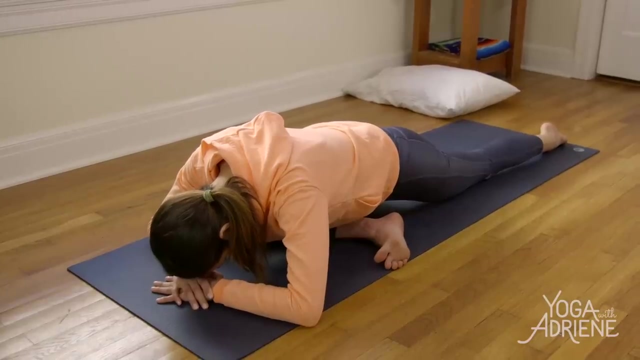 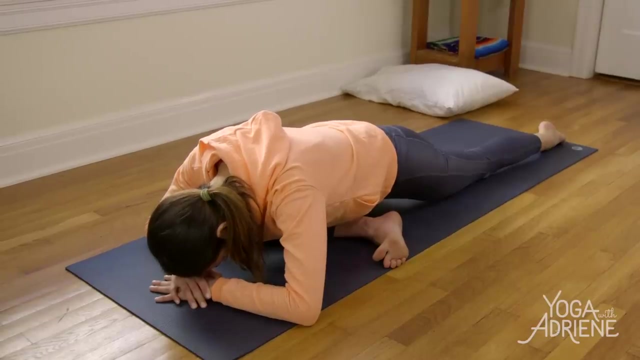 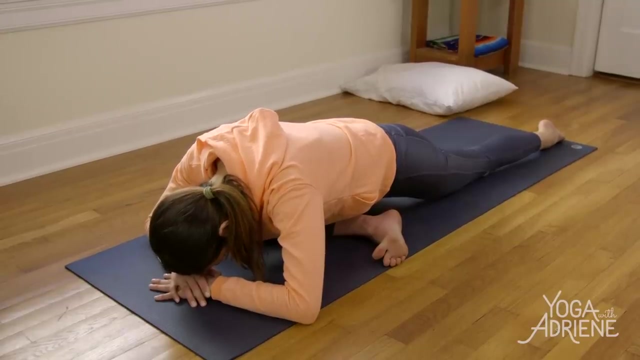 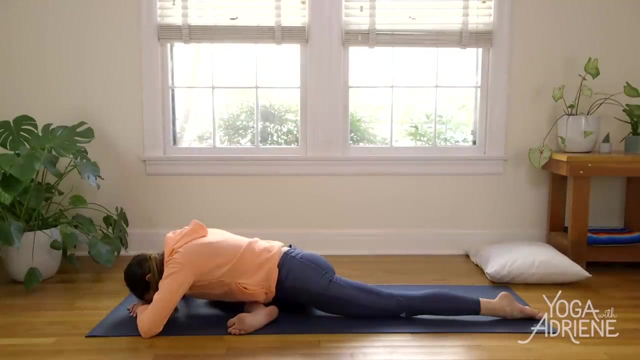 So stick with your breath If you find that you're just like fidgeting and waiting, very normal, natural. so just keep bringing your attention back inward. Great, take one more nice full breath in and out. Then activate navel to spine, connect to your center. 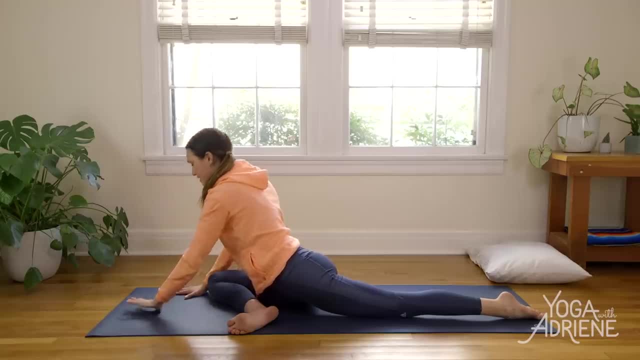 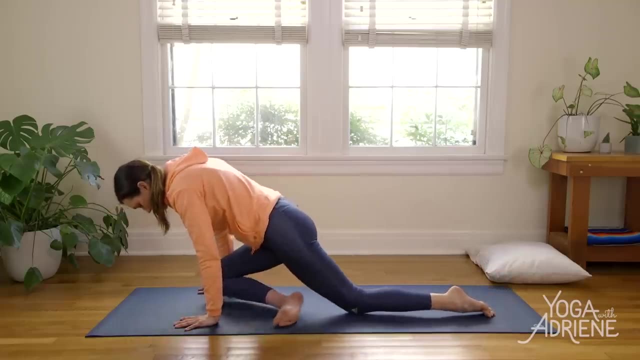 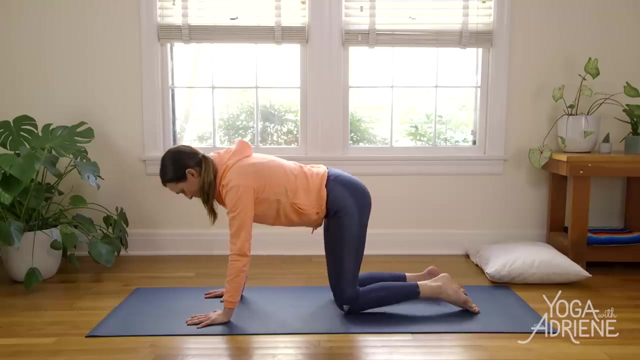 your core muscles and press it up nice and slow. We'll curl the back toes under press in all 10 knuckles, come back to all fours. That same little ditty on the other side. here we go: Big breath in, big breath out. 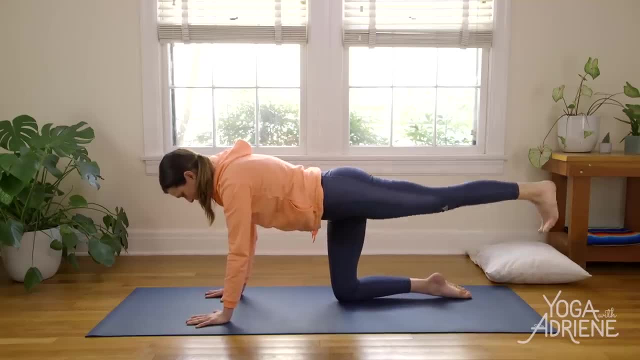 This time send the left leg out. gentle pulses Again. notice if you're collapsing here. can you press away from your yoga mat? This is a nice practice for runners, because when we develop a running practice or a jogging practice or even a regular 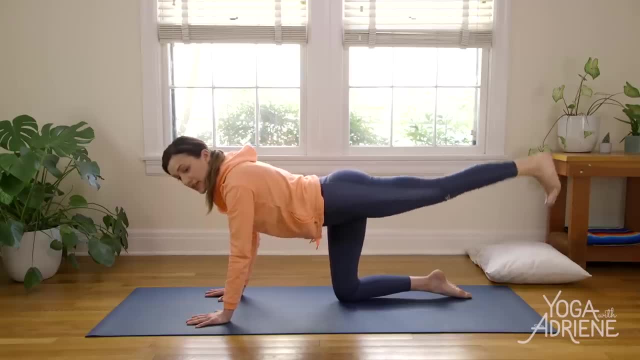 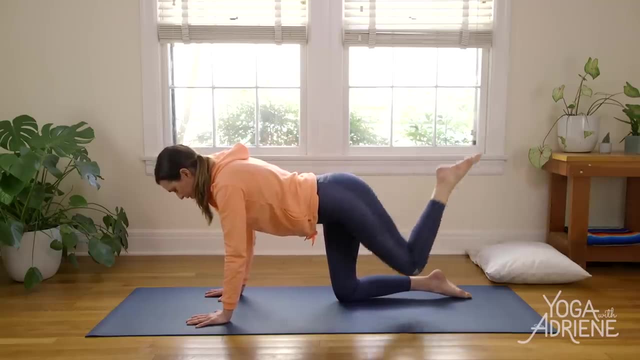 walking practice. we wanna be able to have awareness from head to toe. right one moving part, Then bend the left knee. You can draw it all the way up into your lunge. Keep the right knee on the ground, but you might walk it. 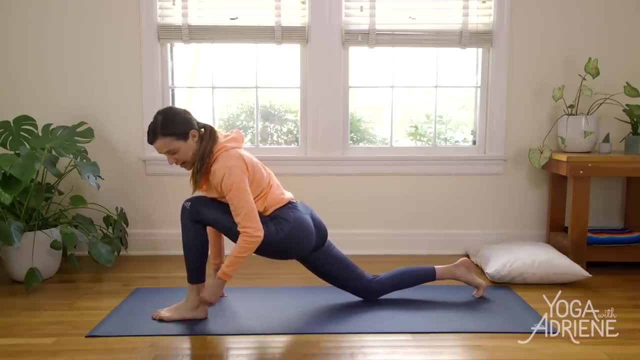 back a little bit and then just check front knee over front ankle here, nice and stacked, Loop the shoulders. stay light on the fingertips. so notice if you're crashing into the fingertips. connect to your core, engage the belly, Breathe. 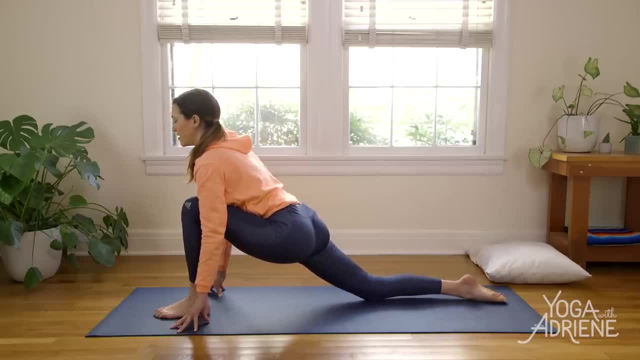 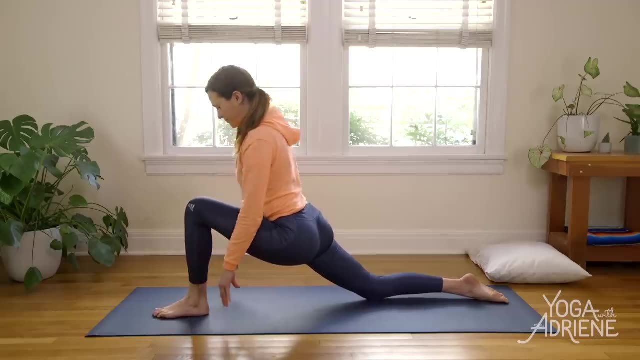 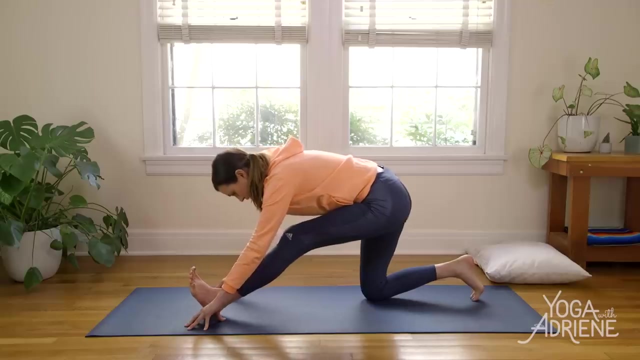 You might come onto the top of that right foot- yogi's choice in that case- Nice- Full, deep breaths And then pull the left hip, crease back, Think up and over as you send the hips back, coming onto the left heel. 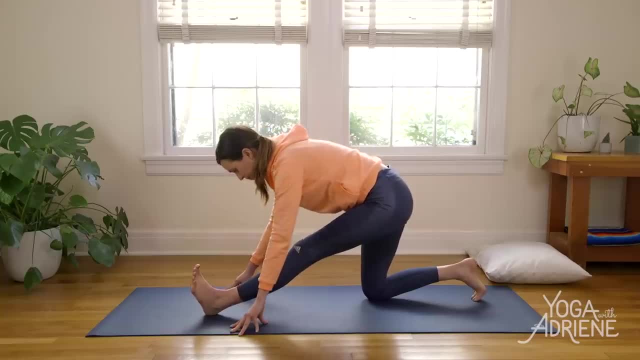 Again. top of the left thigh bone pulls back with the left hip crease, Runner's stretch, big flexion in the left foot. Inhale, Open your heart, find that extension And then exhale chin to chest. So I'd like to point out, notice that my right hip 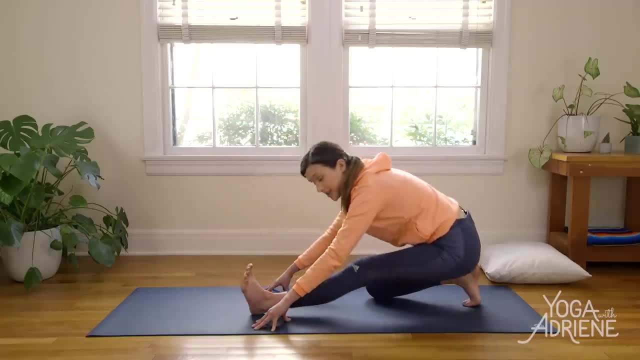 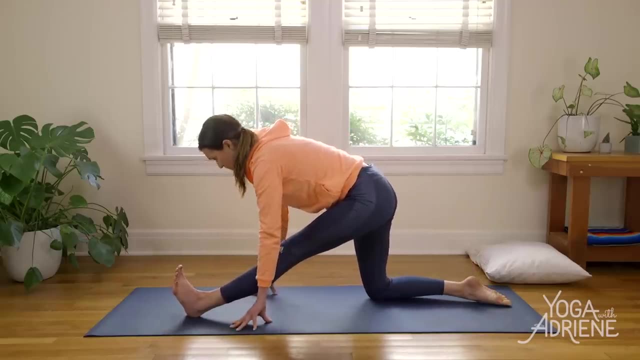 is stacked over my right knee, so I'm not coming all the way back here. So now you're just going to exhale. please hold for a few more seconds and then come back over your left hand to your left and inhale with the left. sebelé. 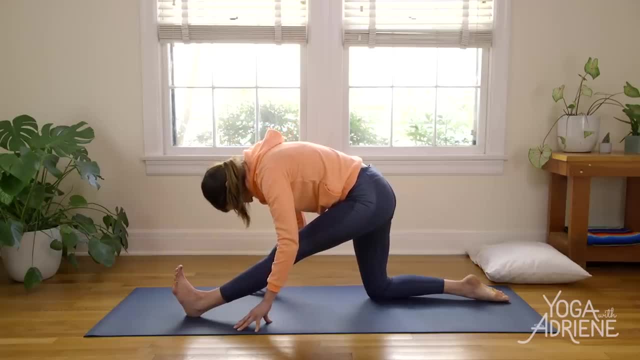 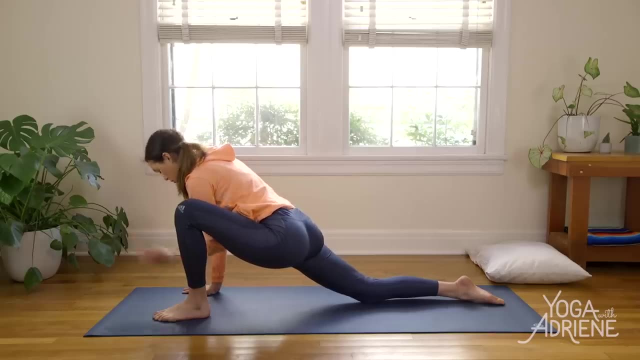 So now our big toe is here, Inhale, Exhale, Inhale, Exhale And then bringing the left hand around, coming into our lizard on the other side. Keep the toes pointing forward here for now. 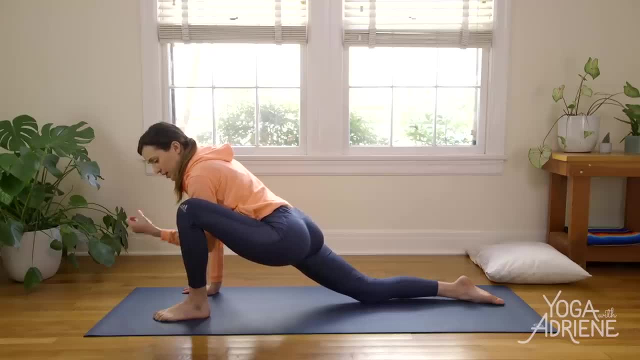 and then notice if you're gripping in the toes. It's kind of a you know, As we begin to open the hips, other things want to clench and so we're going to stay mindful and try to keep an awareness Softness through the toes. 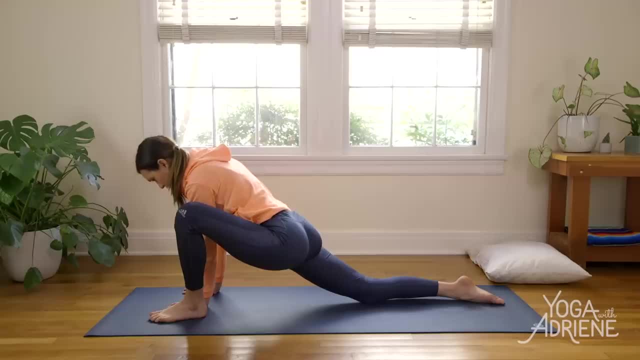 the toes, even the jaw, here. Find extension, Breathe, Pull the left hip, crease back, Give yourself lots of space, So maybe walking that left foot to the outer edge of your left side of your mat, Big breath in, and then you know what to do here. 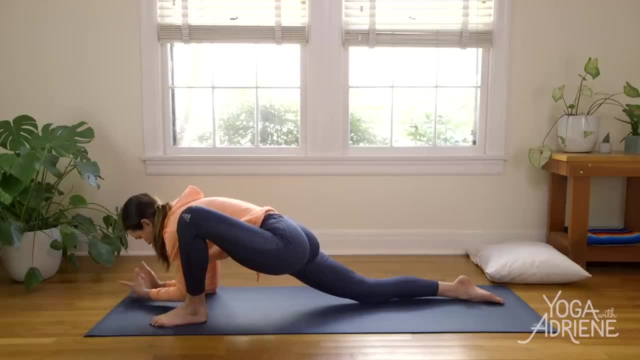 Maybe use an exhale to come onto the forearms. Maybe you save that for another day. Work mindful, Stay connected to your breath And then eventually we'll walk the left toes out and off the left edge. Breathe deep here. 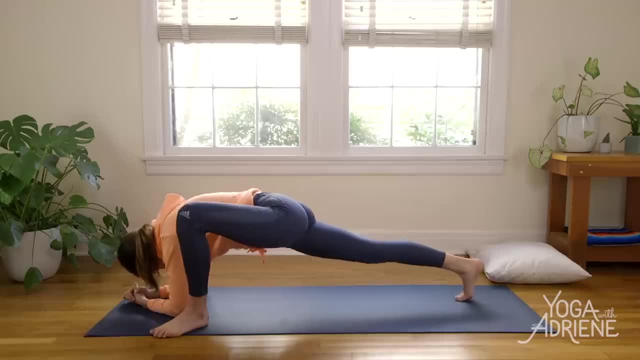 Again, you're welcome to curl the right toes under and spike the right heel back. If you do really spike the right heel towards the back edge of your mat, Really brighten up through that left leg. So keep the hips lifted, engage your core. 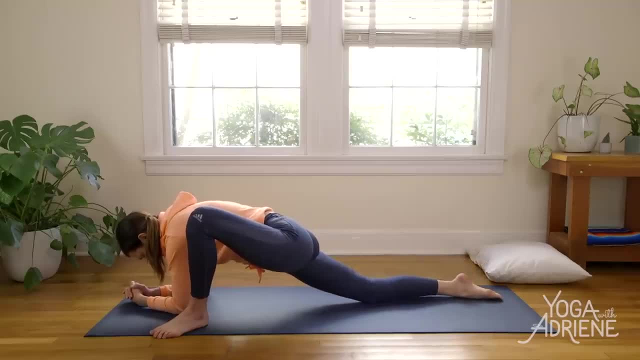 Otherwise, keep it nice and easy Again: allowing for the release today, Allowing for the body to restore And allowing for the practice to balance out your cardio or your other workout- Zumba- And then connecting to your core to release. 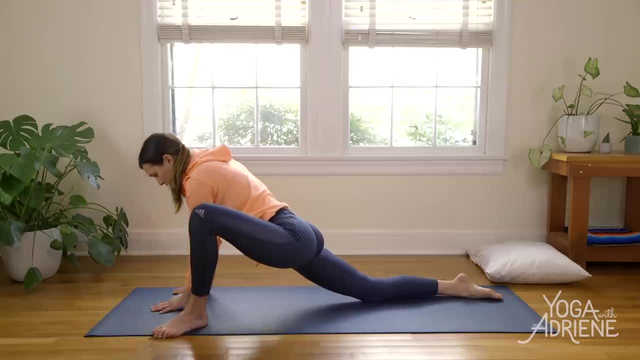 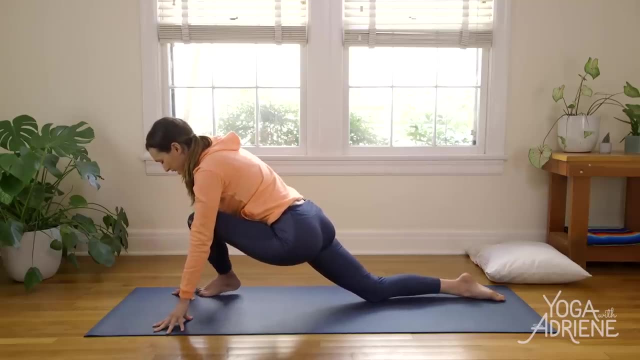 Pressing back up into the core And palms. So even in our transitions we're trying to create a full body experience, Super important right, And then walking the left foot over into our one-legged pigeon. Take your time. take your time. 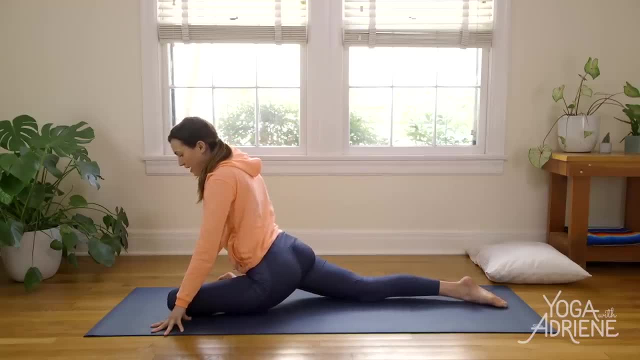 So your pigeon might not look like mine. You might need a little support on the left hip here. You might need to draw your left heel really close into thy crotch, Really mindful. if you're in need of any of these poses, we have a foundations video for you. 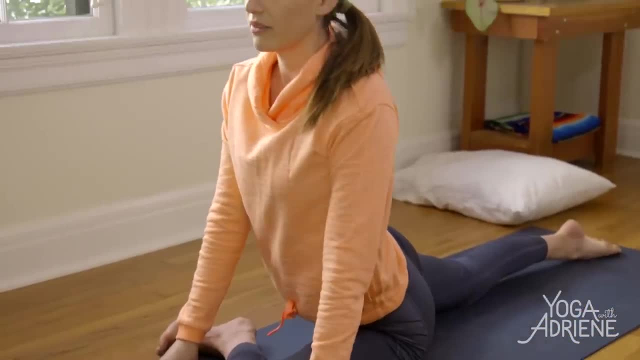 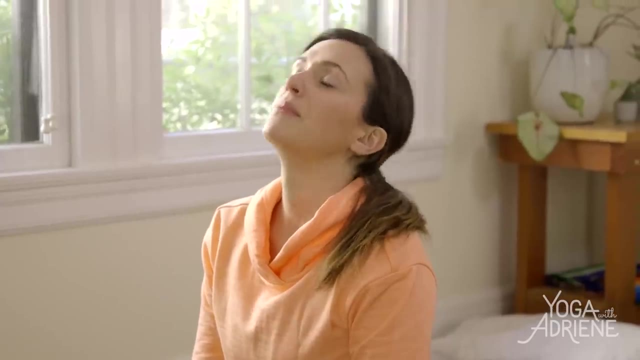 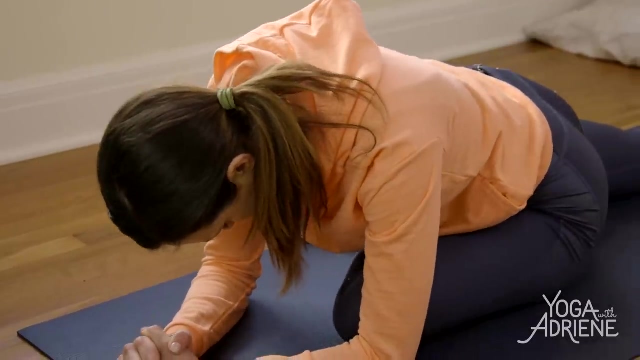 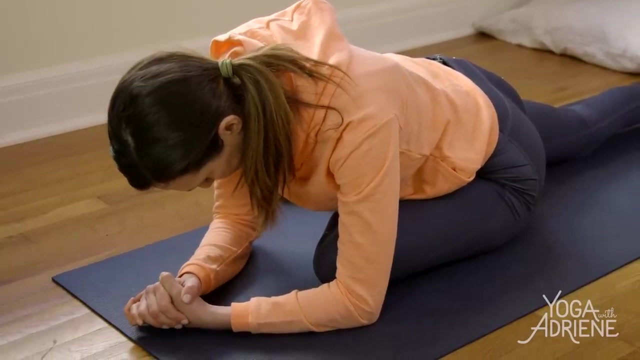 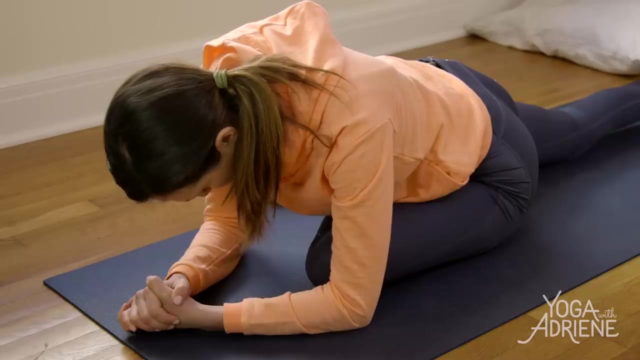 For all of them. So those videos really break down the postures and give you modifications. Inhale, lift your heart, Exhale, find a fold. Everyone stick with your breath, Inhale and exhale, Exhale, inhale and exhale. 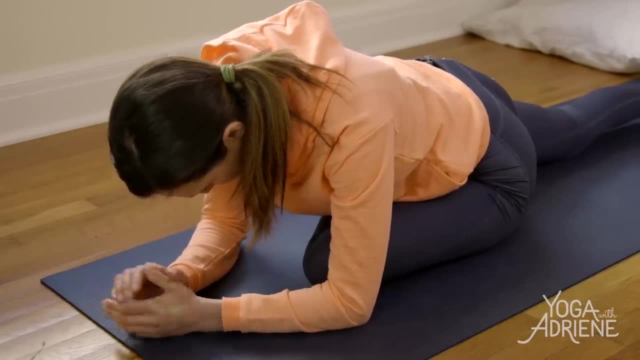 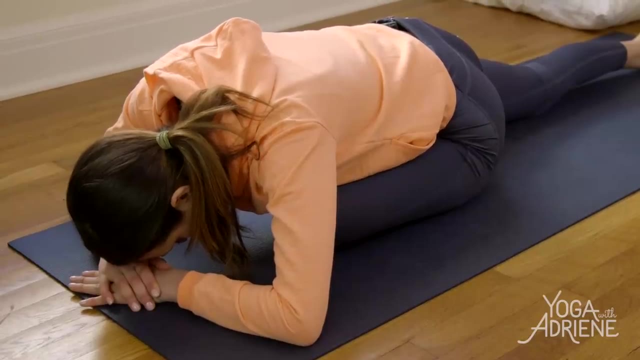 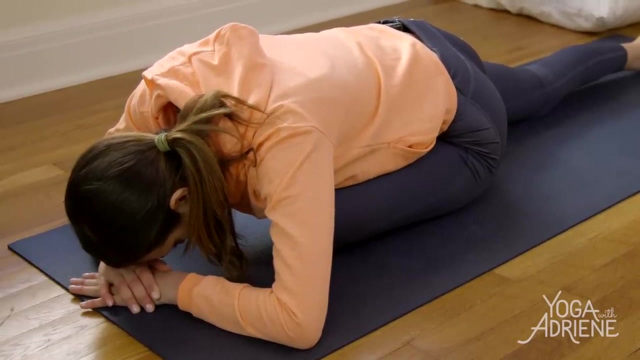 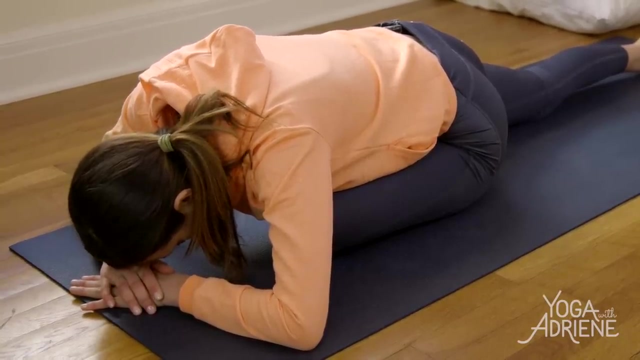 Exhale, exhale and exhale, Exhale, inhale and exhale, Inhale and exhale, Exhale, inhale and exhale ыв, And then slowly connect to your center, press into the palms. 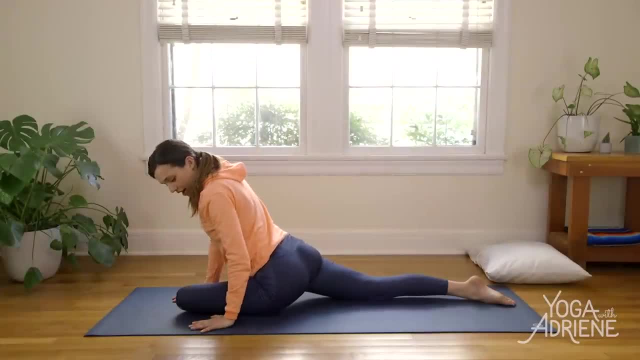 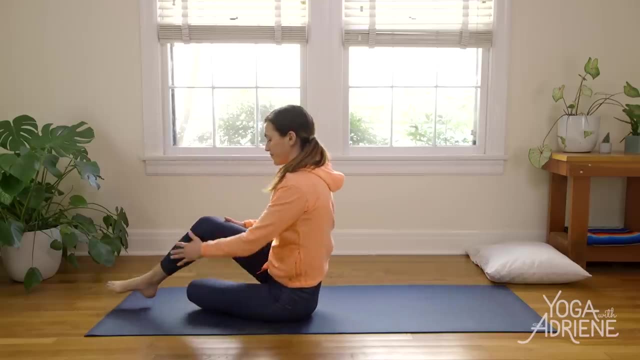 Come back up This time. go ahead and roll onto that left hip. We'll take the left heel in and swing the right leg around. Sole of the right foot comes onto the ground, so there's a tendency to just kind of let it spill here. 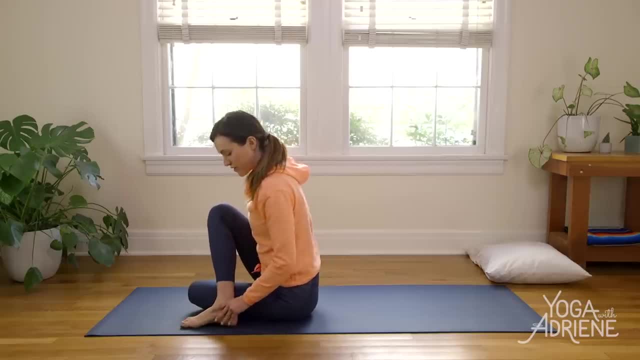 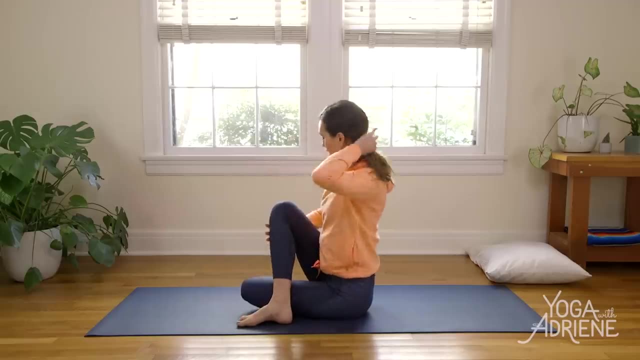 See if you can work to get the sole, all four corners of the feet, on the ground. This might take time. And then a little twist: here I'm going to hug the right knee with the left elbow And swim the right fingertips all the way around. 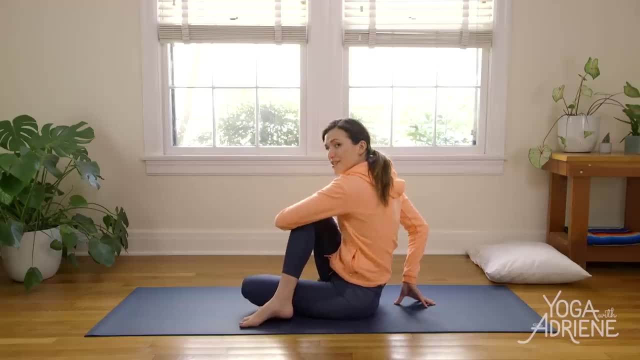 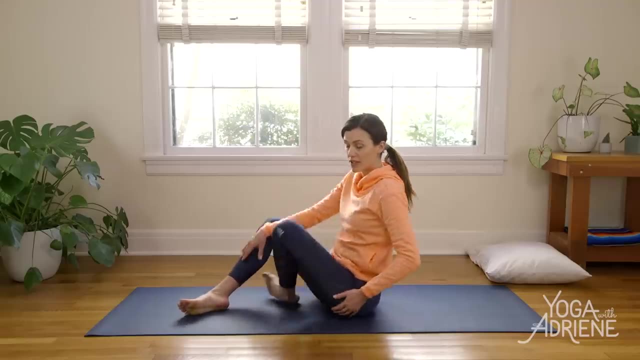 Try to keep a nice big lift in the heart here, Careful not to round through the spine. Inhale in And exhale release. Great, we're just going to switch the legs here, so right heel comes in And we cross the left foot up and over. 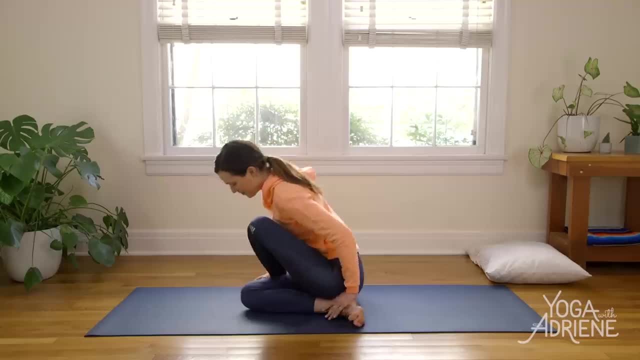 Again. see if you can work to get the left foot all the way on the ground And sit up nice and tall, Hug the right elbow around the left knee And then swim the left, Swing your fingertips around. Just a little twist here to release the back. 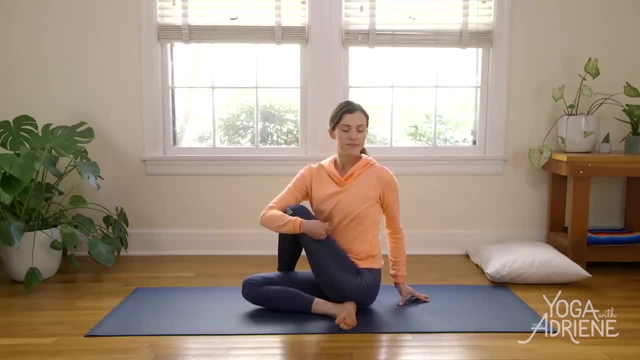 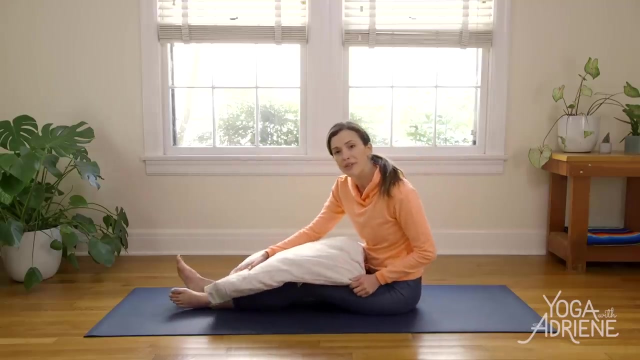 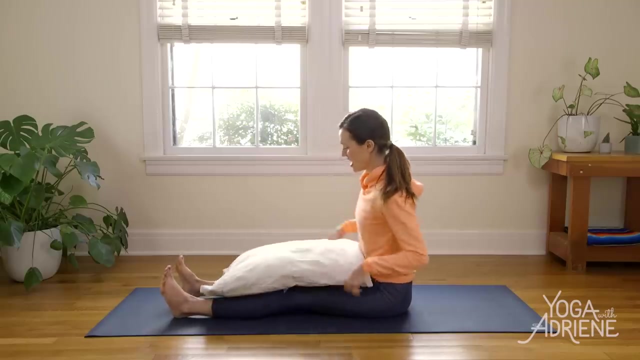 Breathe into your belly, Relax your shoulders And then release And grab your pillow. Yes, This is my actual pillow. This is not a prop. Legs out long, Legs out long. That's going to be okay. no, 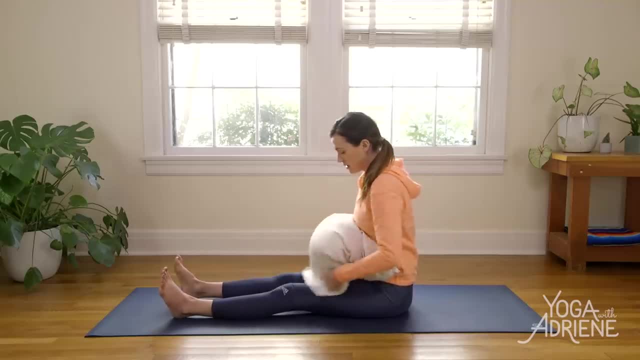 Pillow comes right up to the navel here, So if you have a soft pillow, like this one is, you might even double up. If you have a bolster, you can use that too. I have two bolsters, but I like to use things. 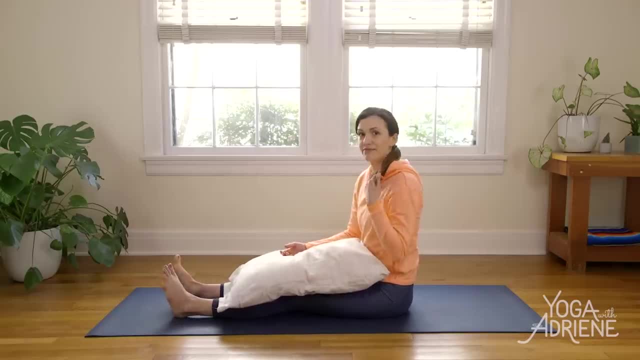 that you have in your house to really promote. you know this idea that anyone can do this And that this is something different than what we do at the yoga studio. I love the yoga studio so much. My life is so rich because of the community at the studio. 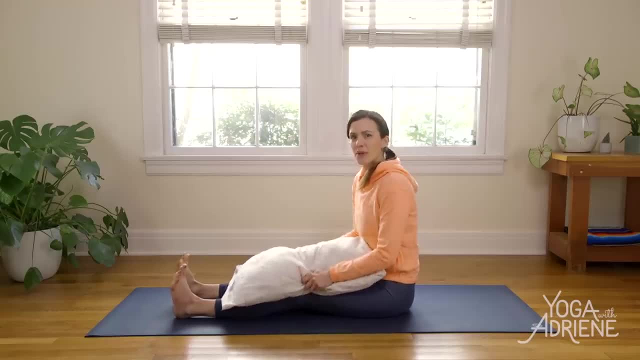 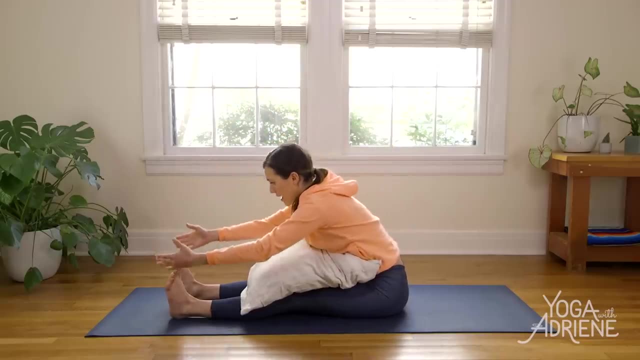 and stuff like that. But this is something different. So own it, Grab your pillow, Pull it up to your belly, Inhale, Reach for the sky And exhale Forward fold. Oh yeah, Same thing as we've been doing all practice. 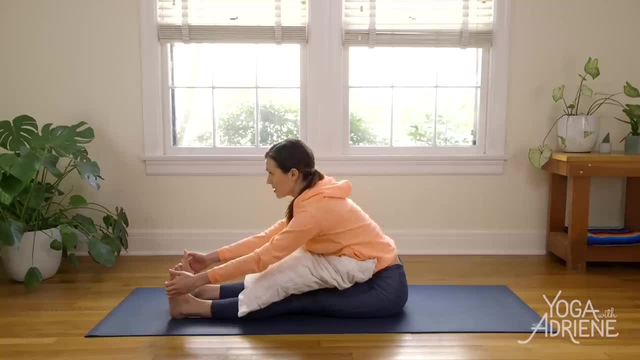 Find that lift in the heart first. Find extension, Inhale Big breath in And after your extension we round forward. Chin to chest, Fold, Release, Close your eyes. here We're going to be here for a couple of nice long, beautiful. 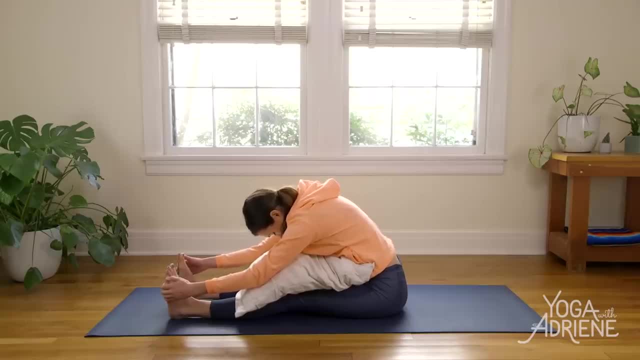 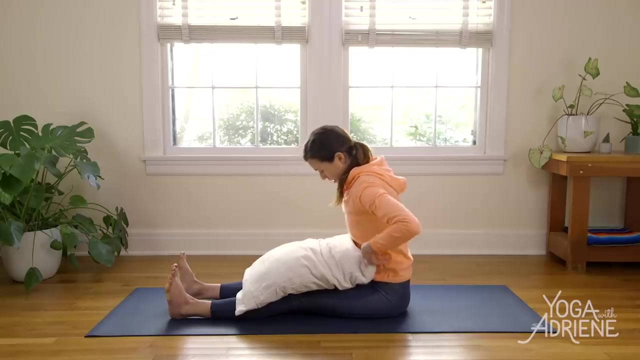 self-loving breaths, Cultivating a little peace in the body, Restoring Great for the nervous system here. So the hands can grab the ankles or the toes here, or you can go full, soften and just kind of release wherever it feels good. 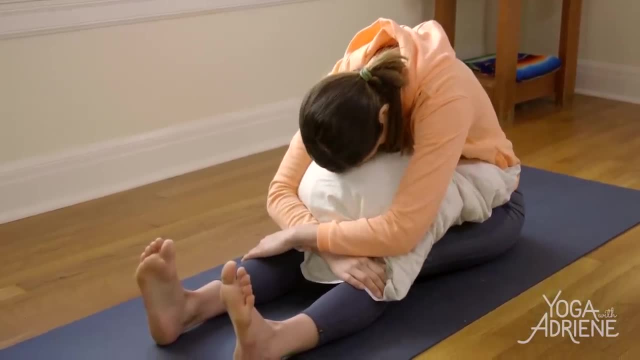 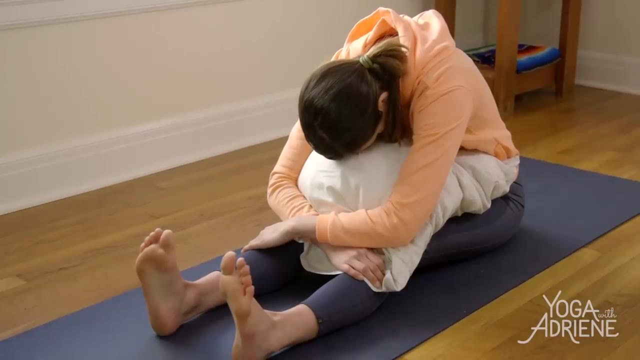 Maybe grabbing your pillow even, And up And down, Come in And out And out And in And out And in And out And out And in. I'm going to take the pillow, slowly roll up through the spine, just slide the pillow. 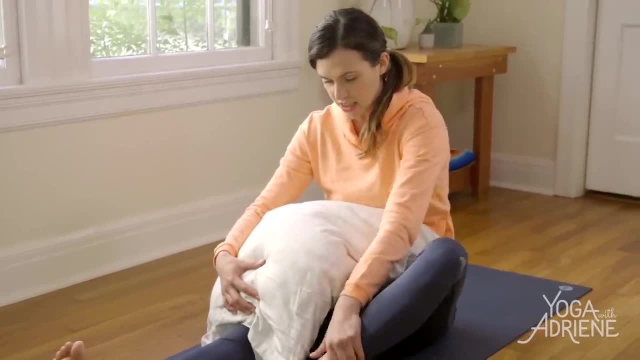 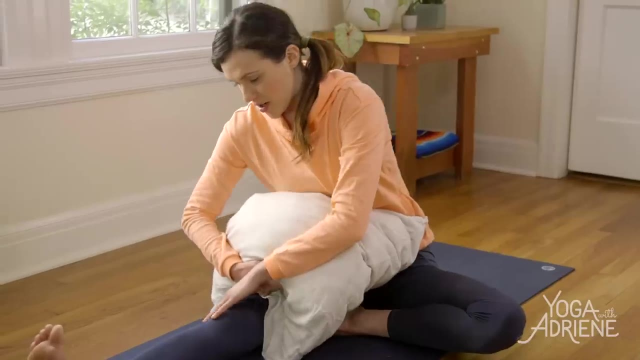 over to the top of the right thigh and we're going to draw the left heel in just a quick Janu Sirsasana, So pressing into the sitting bones, and I'm just going to kind of think up and over as I fold over the top of the right thigh. 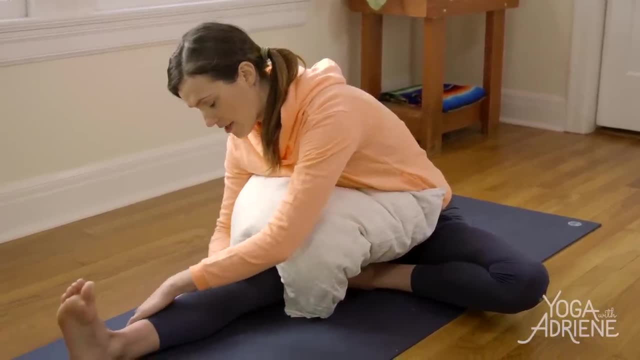 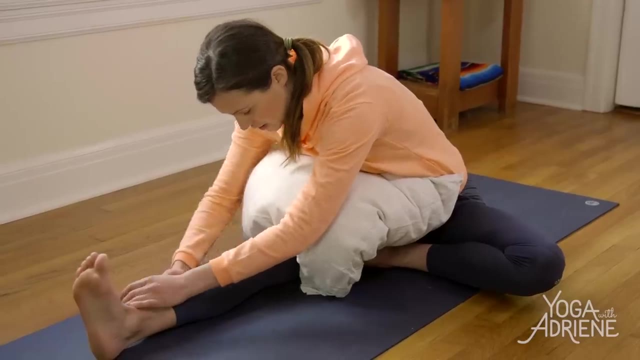 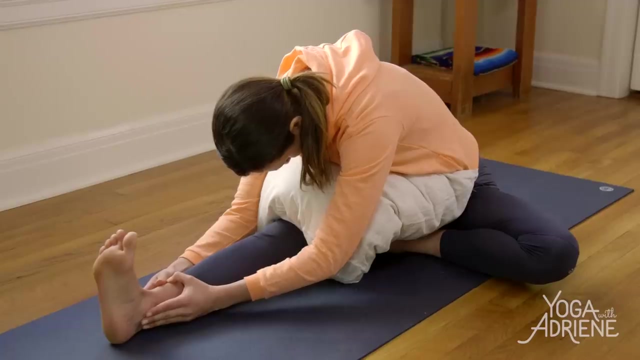 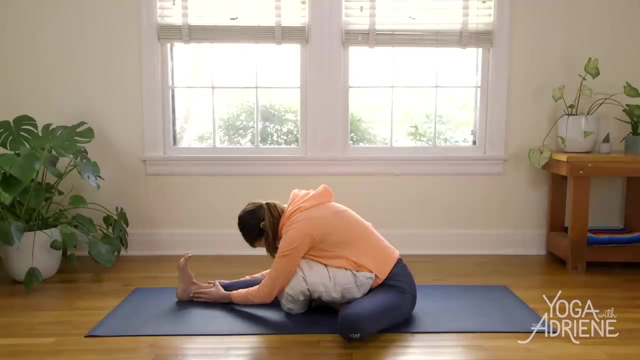 The difference here is I'm going to grab the hand. I'm going to take the hands and grab the outer edge of my right leg, first breathing into the left side body, left hip, and then eventually you can flatten out Head to knee, pose here with the pillow and then slowly roll it up. 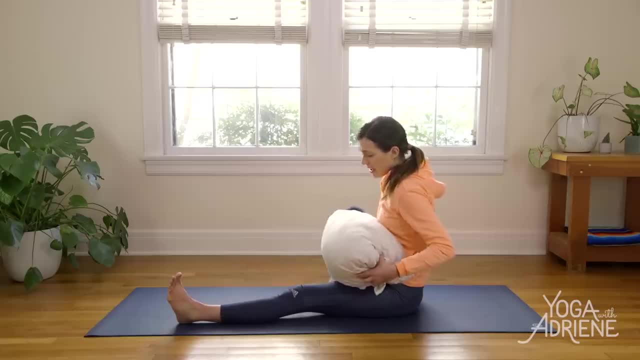 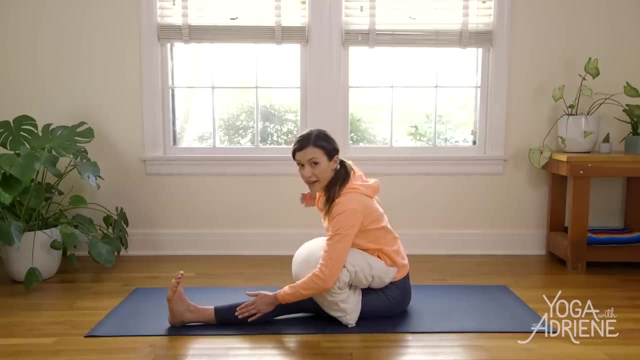 Switch the leg, slide the pillow to the top of the left thigh. right heel comes in and you know what to do: Think up and over top of the right thigh, grounding down. So today's sequence is a great one to learn. 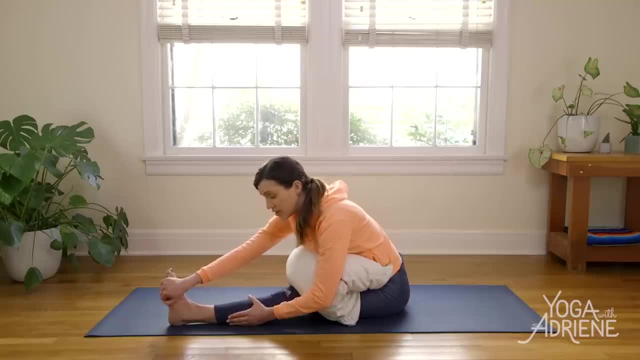 You can favorite this video so that you can repeat it regularly, and then eventually you'll get all of these in your mind bank, in your body bank. As much as I want you to do it with me, I definitely just want you to have these tools inside eventually flattening out. 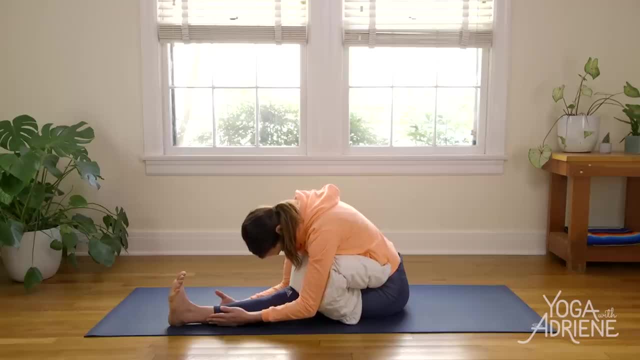 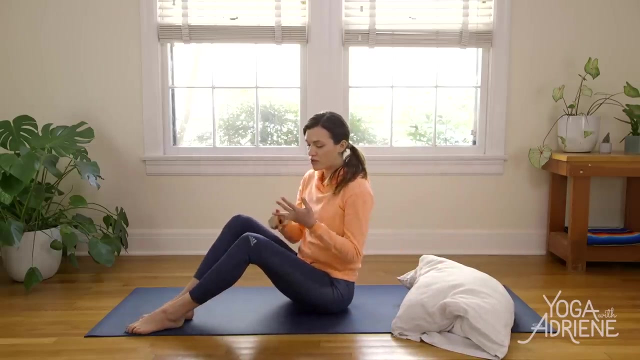 Head to knee pose and then we release: Awesome. Take the pillow, bring it around, use it for your head If you're running or walking or jogging or anything like that, and then also balancing it out with yoga. you definitely deserve these next two pods. 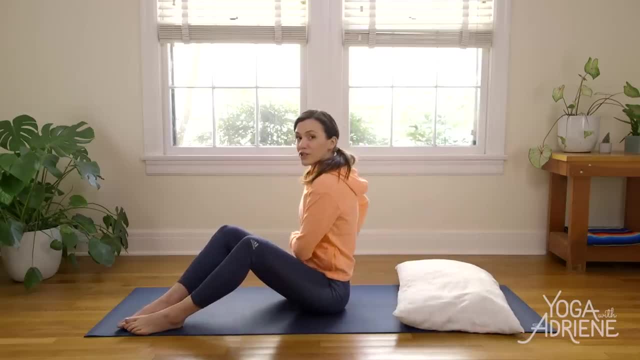 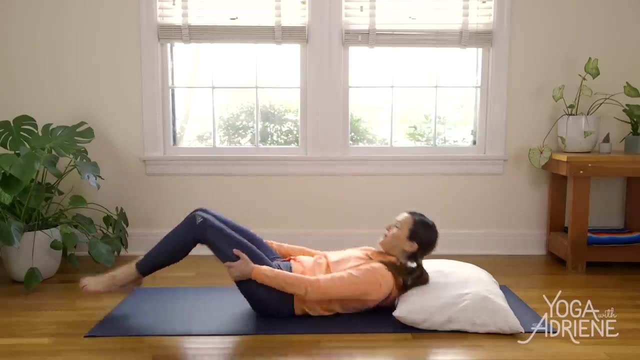 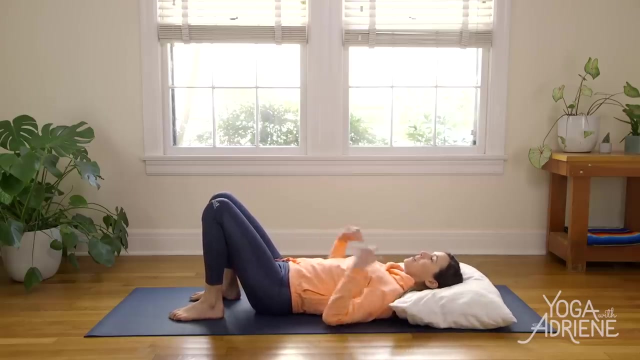 So you can do these postures with a pillow, Way to show up for yourself, Way to keep moving, right. So come to lie flat, Use your pillow wisely, Get comfy And then hug the knees into the chest. Almost done here, guys. 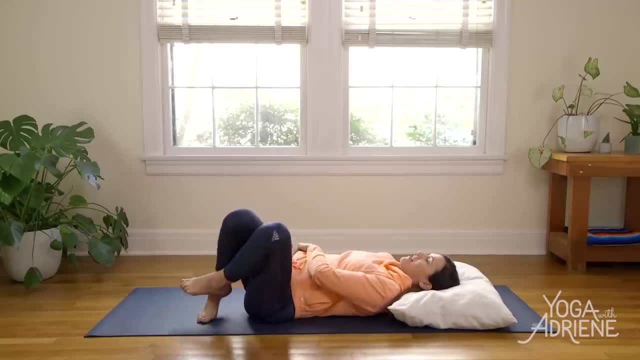 So nice, strong, full, deep breaths. Make them count because you're worth it. and this is only going to help us when we get back. But you know, in our running shoes get back on the pavement, So squeeze the knees up towards the chest, give yourself a big hug, roll around a little. 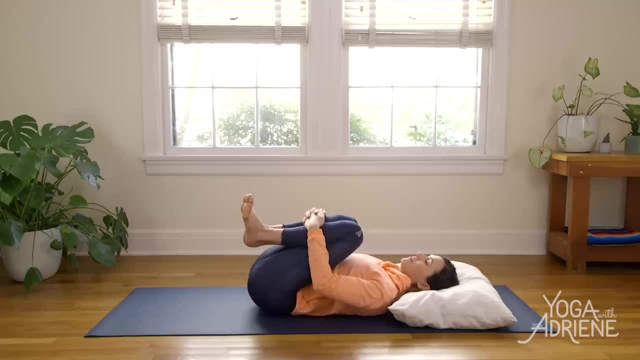 bit and then happy baby pose. So we reach around, knees go wide and we grab the outer edges of the feet and we draw the soles of the feet up towards the sky. So there's really an activation here: lifting the soles up. 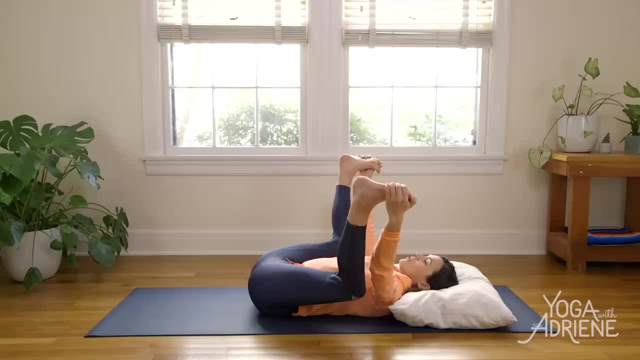 And then grounding down through the shoulders, through the knees, Action point: Lengthen the tail, bone your coccyx towards the front edge of your mat And then breathe into all four sides of the torso. Life is good. We're so lucky to have these bodies. 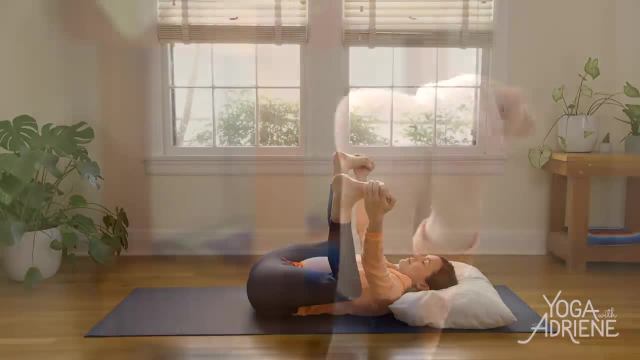 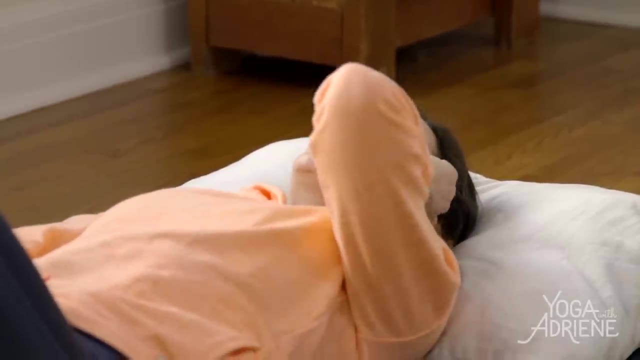 Give thanks for your body, for your breath, And then gently release soles of the feet, come to the mat And we're going to turn onto feet. We're going to turn onto feetal position, whatever side is towards the video here, towards. 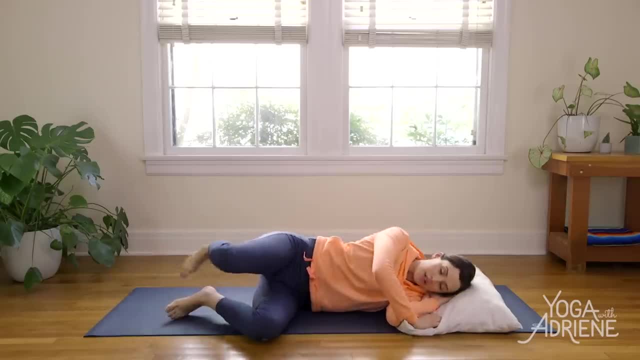 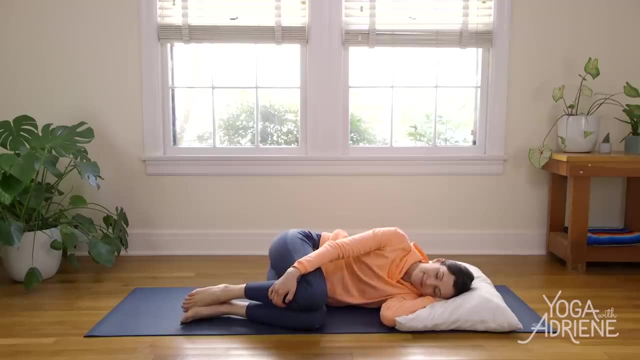 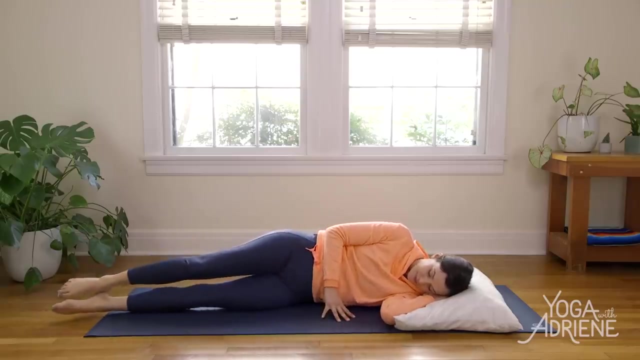 the screen. So your bottom arm becomes a little pillow. with your pillow The knees hung up, nice curvature in the back body, just a little release for the spine. And then, last thing: before we rest, we're going to send the legs out long. 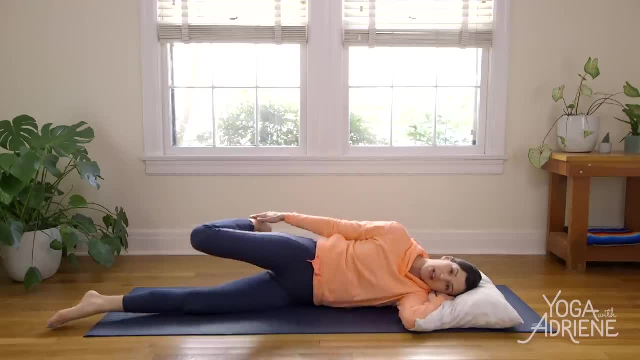 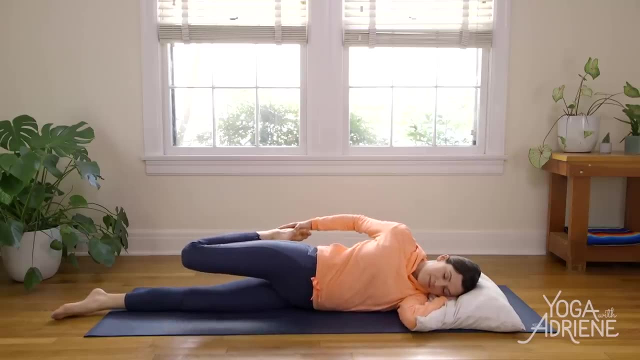 And top knee is going to bend, Top arm is going to reach around and grab top ankle and we come into a little quad stretch. here You can roll onto your belly for this if you want more Breathing into the quads, opening up the quadriceps, opening up through the chest and 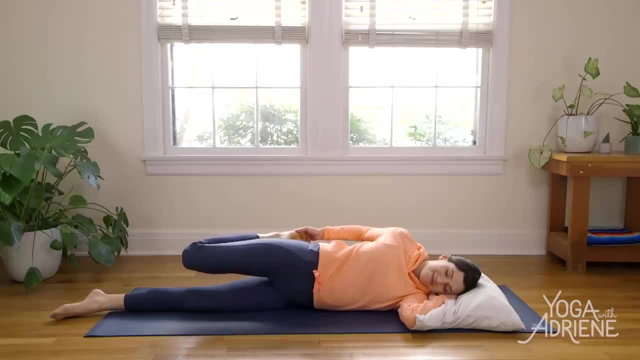 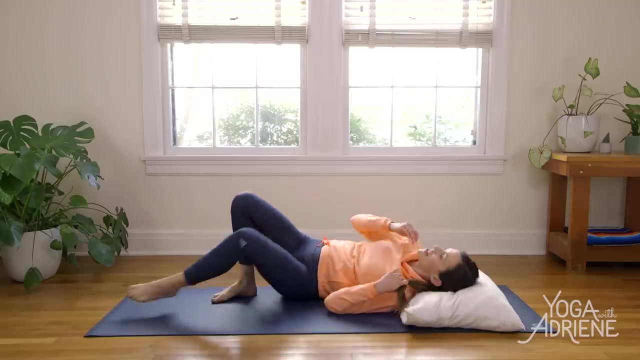 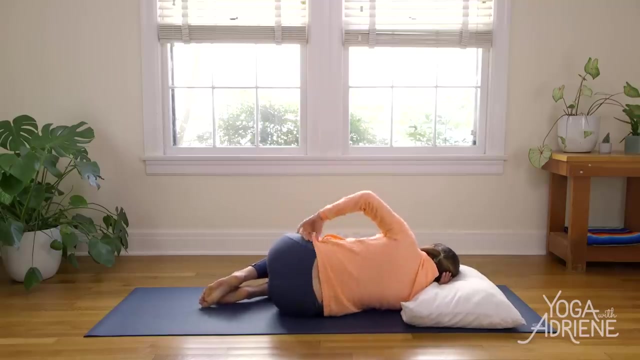 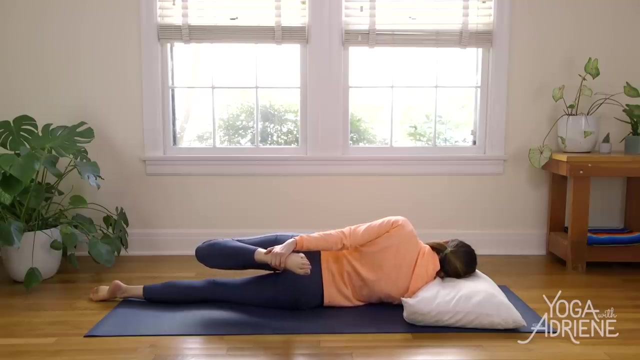 the heart here Again. you can also do this on the belly Sweet And then gently release Rock onto the other side. Take that feetal position first- it's nice- and then extend the legs out long Top knee bends, grab top ankle quad stretch on the other side. 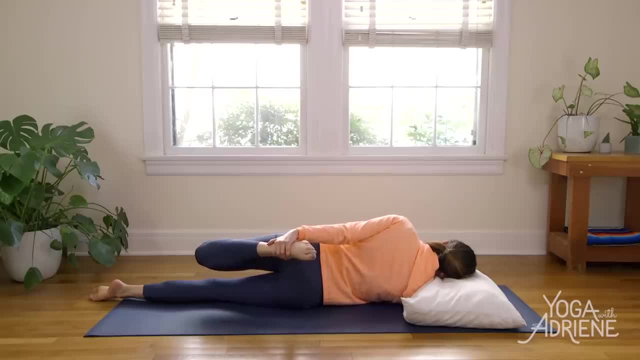 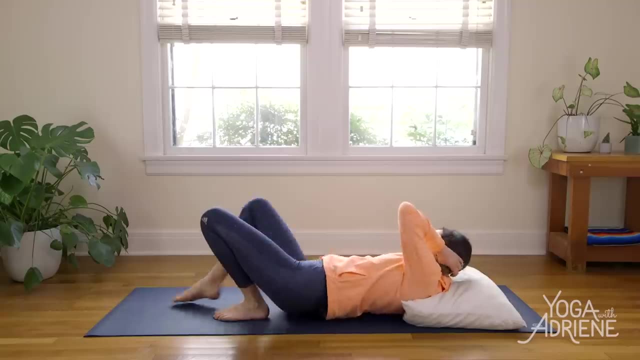 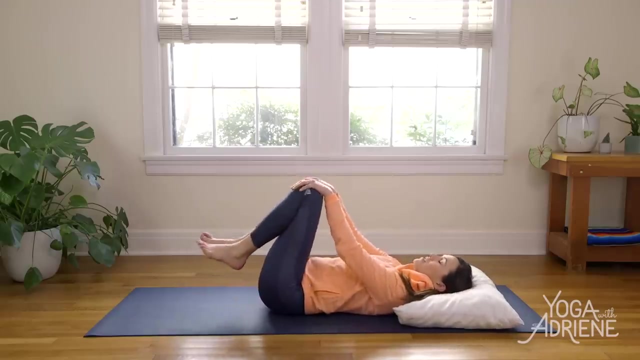 Where's your breath? And gently release Good, Good, Good, Good, Good, And release, Roll back onto your pillow Palms, come to the knees- Little release of the back here, as you just gently reach the knees towards the front. 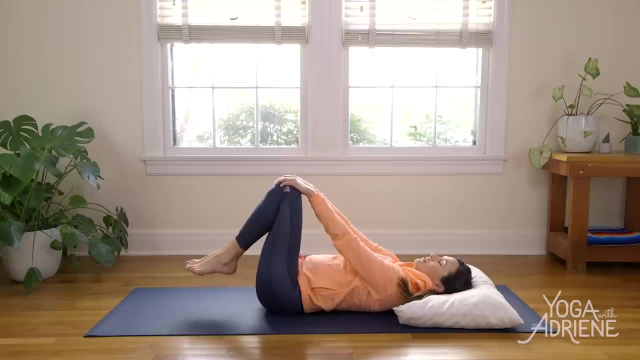 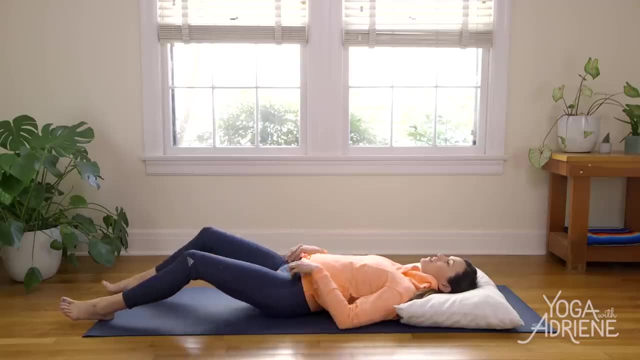 Arm straighten here, Very gentle stretch, And then let it all go. So you're either going to extend out into savasana now or you're going to close your eyes for one final breath before the video starts. Good, Good.